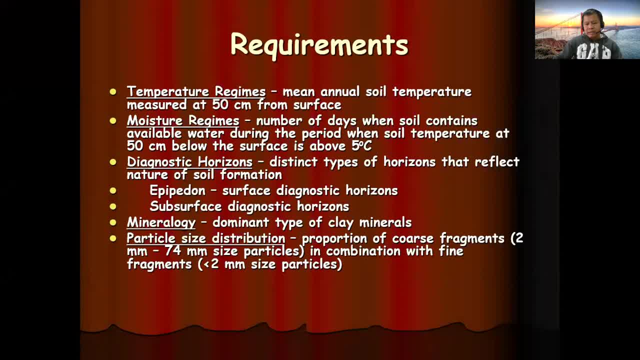 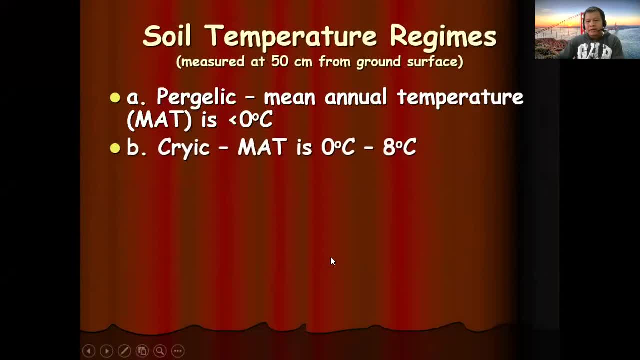 What is on the A horizon? What is on the subsurface horizon, Mineralogy, particle sizes. Now let us look at first the soil temperature region. So what are the different soil temperature regions in the control section, measured at 50 centimeters from the ground surface? 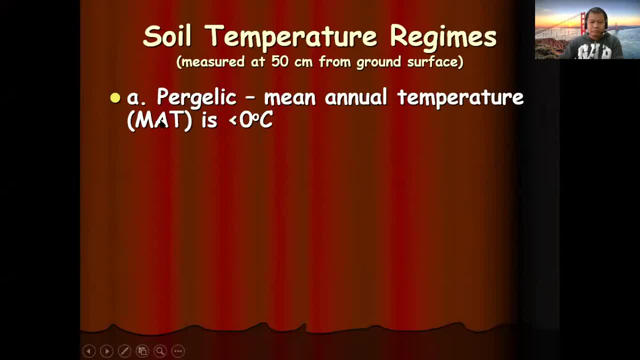 Okay, So we have what we call pergillic. One of the soil temperature region is pergillic. So what is this? The main annual temperature, measured at 50 centimeters from the ground surface, is less than zero degrees Celsius. 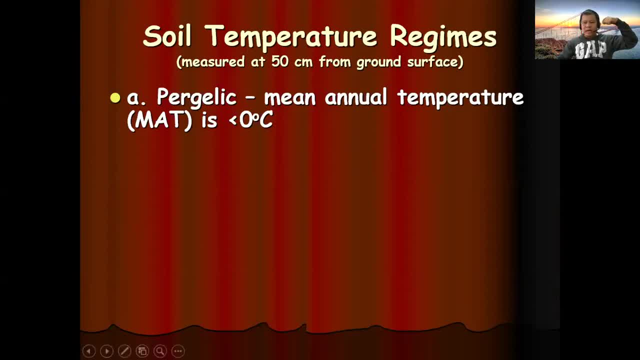 So look at this sign. It's less than Dito sa left side ng ating braso is less than- and this is greater than Sa to greater than less than sa, wala, All right, So pergillic. the main or the average yearly annual temperature at the control section is less than zero degrees Celsius. 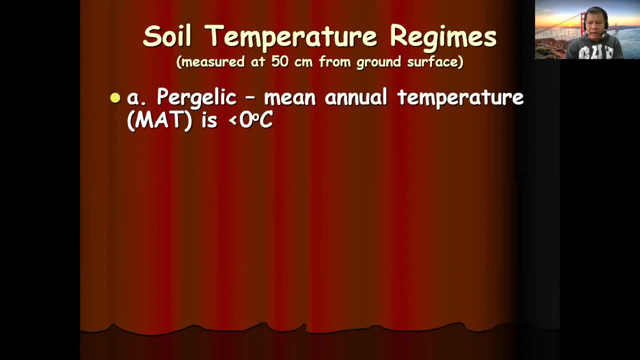 Kapag kinuha natin yung temperature Doon sa critical control section, which is the measured at 50 centimeters from the ground surface, Pag less than zero degrees Celsius ang average annual temperature ng section na yun. that belongs to a pergillic soil temperature region. 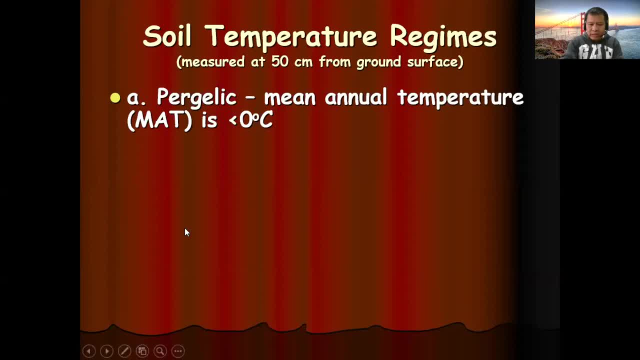 So take note for that Pergillic. less than zero degrees Celsius, Maybe negatives, They are negative one: No Below zero. Another soil temperature is cryic when the main annual temperature is between zero degrees Celsius up to eight degrees Celsius. 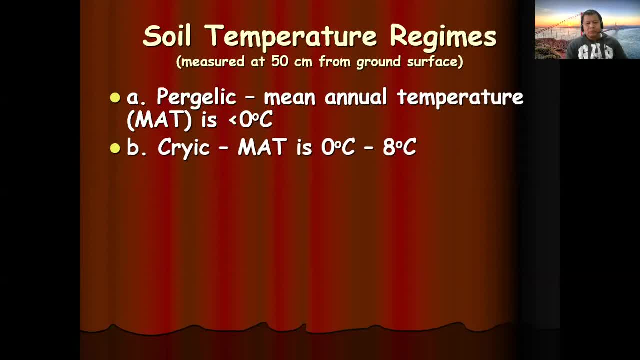 So take note for that. The same temperature from the soil control section. Excuse me Another soil temperature region: pergillic. so when the main annual temperature is less than eight degrees Celsius warmer than cryic in summer. So if it's warmer than cryic in summer, then it is pergillic. 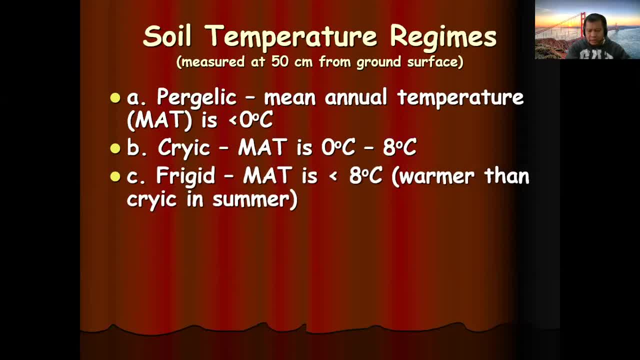 So less than eight degrees Celsius. So basic ang temperature ng control section ng soils if the main annual temperature is eight degrees Celsius and up to 15 degrees Celsius, So yan yan, And another is thermic, or the main annual temperature is within 15 degrees Celsius, up to 22 degrees Celsius. 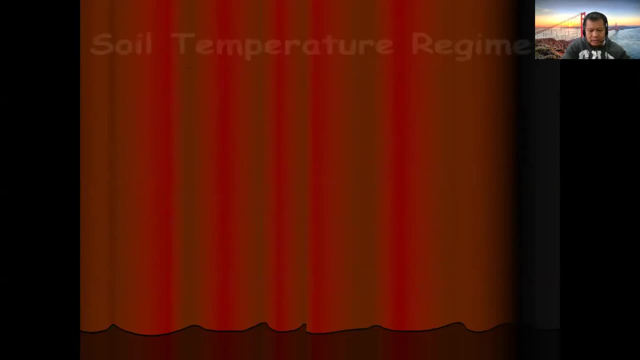 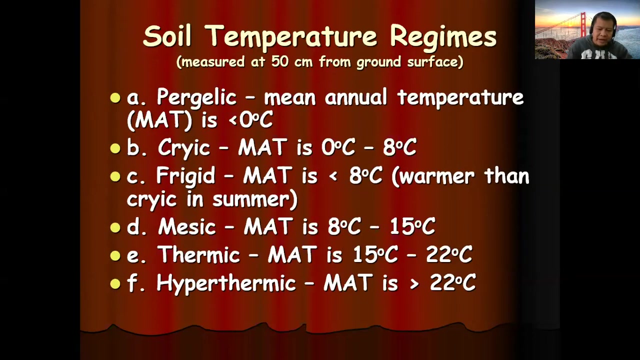 And the last one is hyperthermic. When you see hyperthermic, it is higher than thermic temperature. Okay, So hyperthermic is higher than thermic When the main annual temperature is greater than so. this is greater than sa tuong aside sa kanang bahagi ng ating kamay. 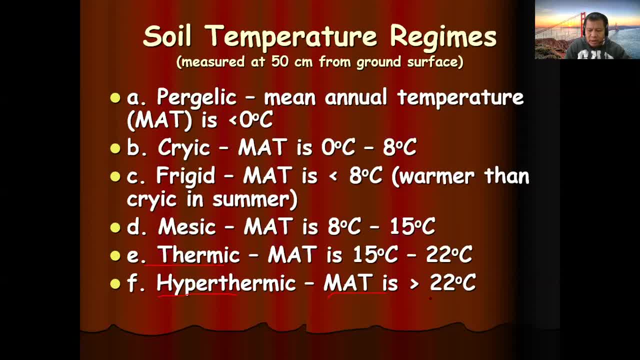 So the main annual temperature is more than 22 degrees Celsius within the control section. Okay, So take note for that. Well, please find your convenient way of memorizing this one in order, So maybe you can have your acronym. 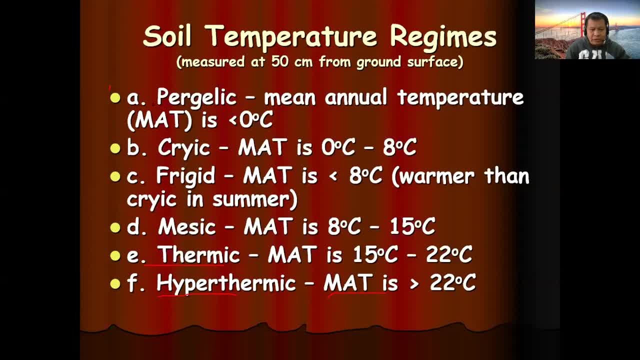 So you can organize your acronym In here. you can do a per- I don't know per per crypt. no, you can do a per crypt per cryptmethyhy. You can do that per cryptmethyhype. 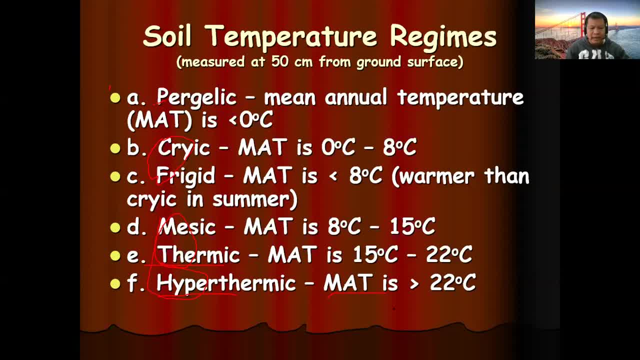 So per cryptmethyhype, So you have pergylic cryic, percrypt, if prigid me mesic t, thermic, hyperthermic, So you can have your own code for that. 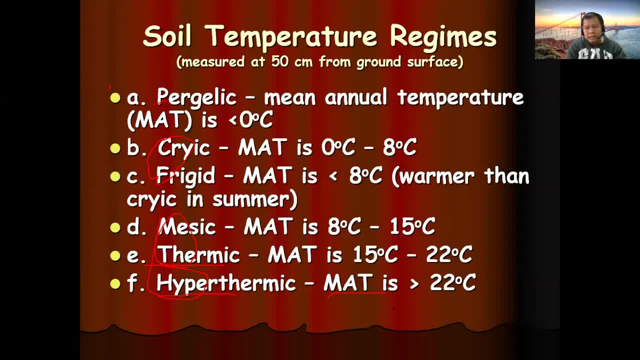 You can have your own. what's this acronym for that that you can decode later on. Because it is important to memorize this one, because, yeah, In previous exam may lumabas na mga ganito, So please memorize this one. 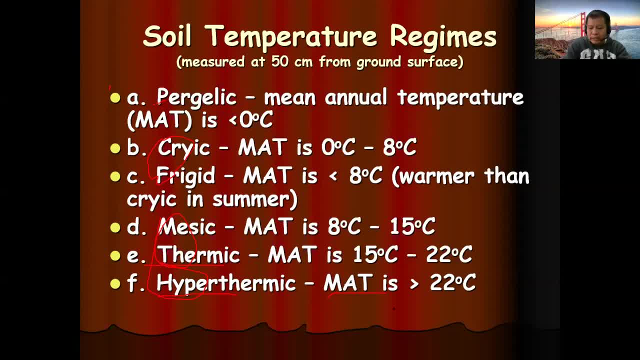 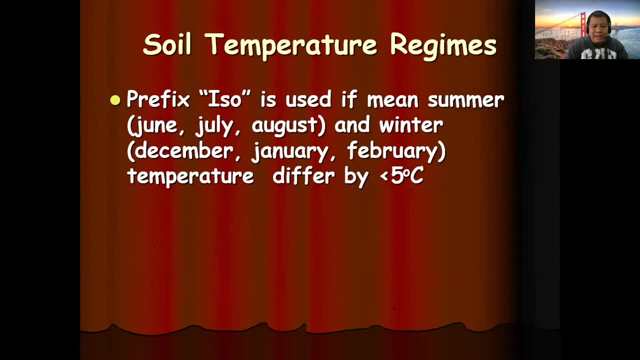 And how are we going to use this one in naming swells Bakita natin later on? Okay, So that is for swell temperature regime. So to continue, So yung mga swell temperature regime na yun, we have to add a prefix ISO. 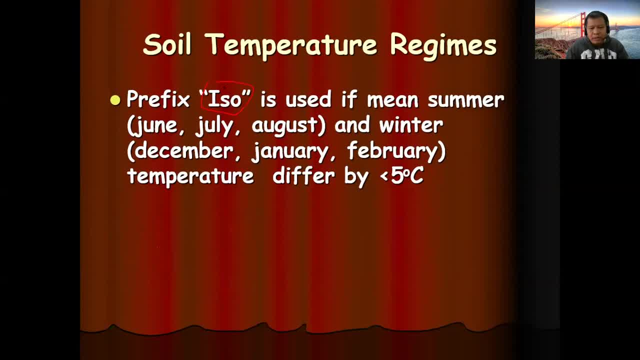 So dagdaganitin ng ISO Prefix. ISO So is used The mean summer. So the summer in the Philippines you have the June, July and August If the mean summer and mean winter, which is December, January and February, differ by less than 5 degrees Celsius. 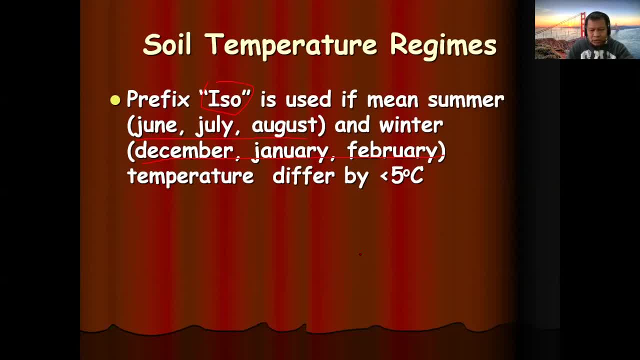 Again you have to use the prefix ISO. So if the mean summer and mean winter temperature differ by less, If the mean summer and mean winter temperature differ by less than 5 degrees Celsius, now in the same control section, kung ang temperature niya sa annual temperature niya sa summer, compared to annual temperature niya sa winter would differ by less than 5 degrees Celsius, then we have to add a prefix ISO. 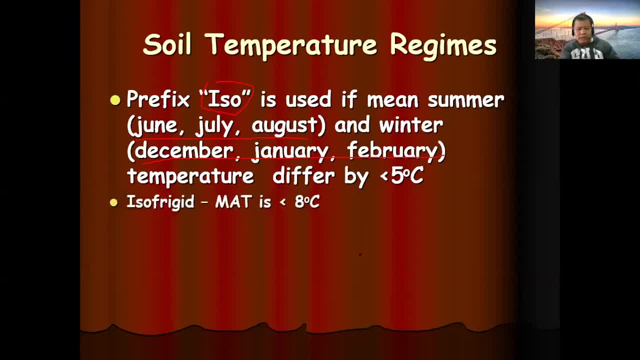 So, for example, so isoprigid, no, So isoprigid, So isoprigid. the mean annual temperature ng isoprigid is less than degrees Celsius within that control section. Okay, Kung nagvari ang temperature ng summer and winter of less than 5,. but for example, 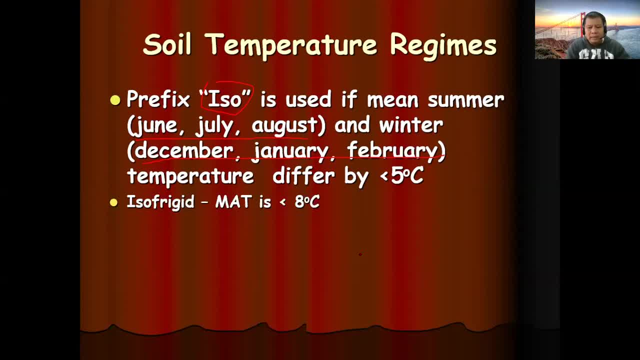 ang temperature ng summer is, shall we say, 5, and then the temperature ng winter is 7.. Therefore, the difference is 5, and 7 is 2, and it's less than 5.. Therefore, ang tawag natin sa temperature regime na yan because it has a difference of less than 5 degrees Celsius between summer and winter. 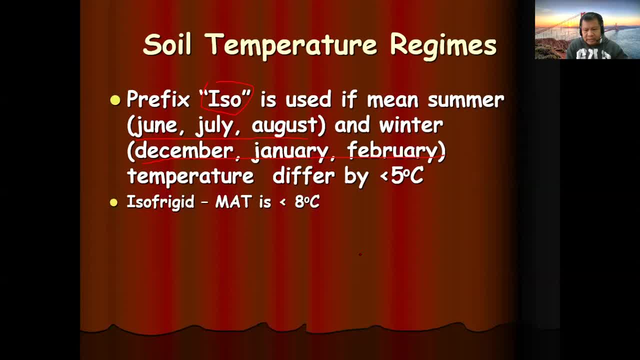 and ang main annual temperature is 5.. So if the temperature is less than 8, tawag natin ang isoprigid. So ganun yan, So ganun din kung MISIC. so ang MISIC is the temperature is ranges from 8 to 15 degrees Celsius. 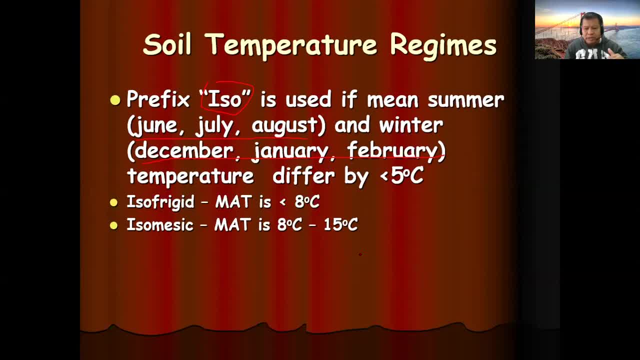 But if the difference between the summer and winter and it falls within 8 to 5 degrees Celsius, it's MISIC. if the difference is less than 5, then we have to call it an isomisic. Okay, And then ganun din: iso-hyperthermic kung the difference between summer and winter of the thermic temperature is less than 5,. 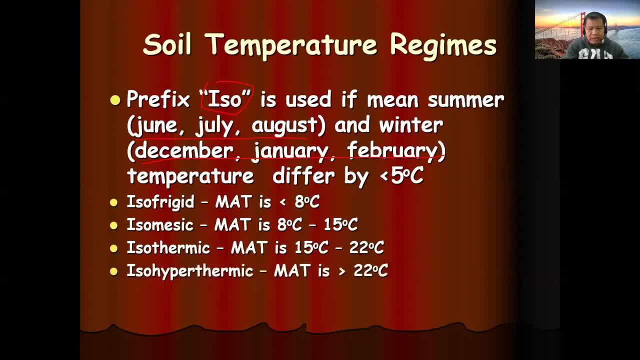 then we call it iso-hyperthermic, Ganun din isothermic, if the average temperature in the entire year is less than 22,. but the difference between summer and winter is less than 5 degrees Celsius, then, sorry, if the temperature of the entire year, an average of that particular control section, is more than 23 degrees Celsius. 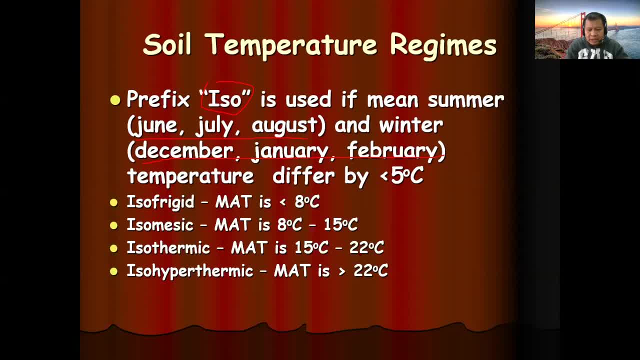 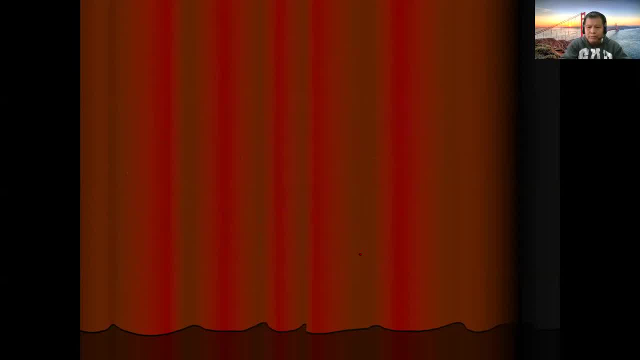 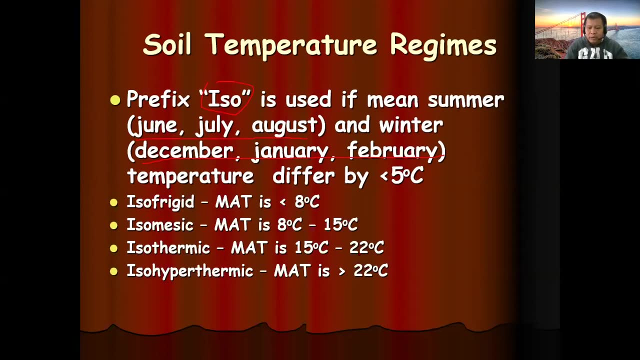 but the difference between summer and winter is less than 5, then we have to call that temperature regime as iso-hyperthermic. So meaning to say all we have to do is just to add a prefix, iso- when the difference between summer and winter temperature 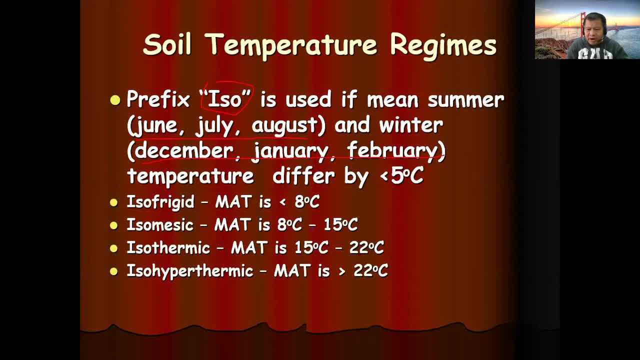 of that particular, of that particular swill, temperature regime varies by less than 5, then we have to add an iso prefix, such as for this particular example. Okay, So please try to understand this one, because Okay. 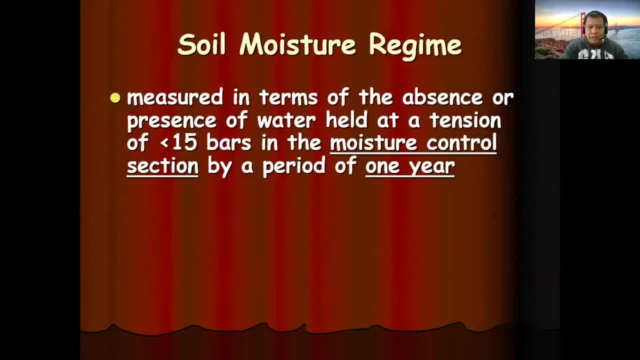 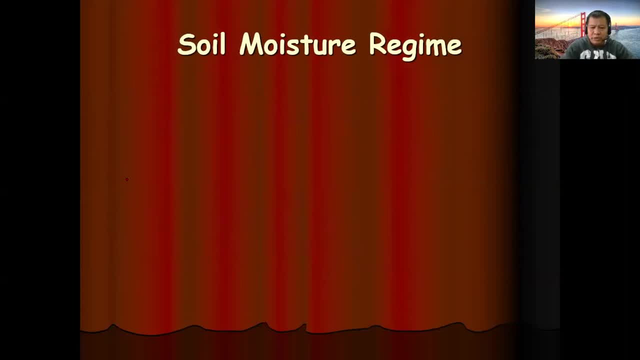 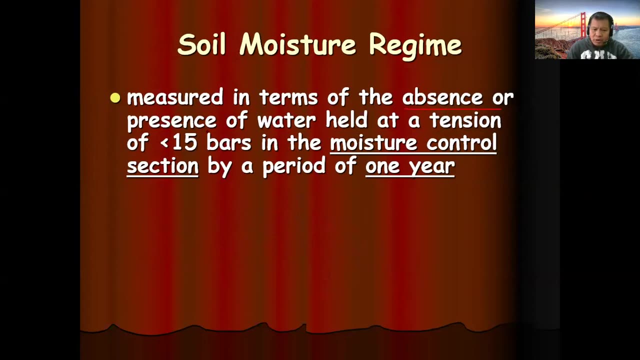 So let's proceed. Okay, So when we have a swill temperature regime, we also have a swill moisture regime. Okay, So what is swill moisture regime? So swill moisture regime measured in terms of the absence or presence of water. 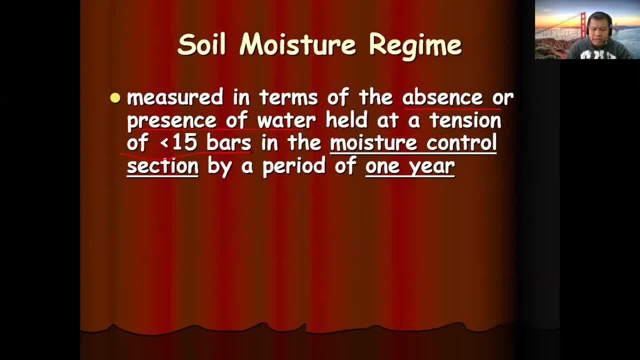 held at the tension of less than 15 bars in the moisture control section by a period of one year. Again, swill moisture region is regime- is measured in terms of the absence or presence of water healed at the tension of less than 15 bars. so bucket 15 bars and I consider because less than 15 bars. 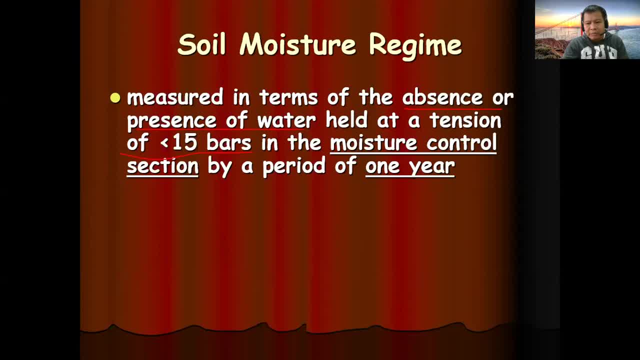 because greater than 15 bars or beyond 15 bars, the roots cannot absorb the soils and the roots can absorb the water that has been healed in the sewer, in the soil surface, or more than 15 bars. So ang kaya ng tanom, ang kaya ng plants to 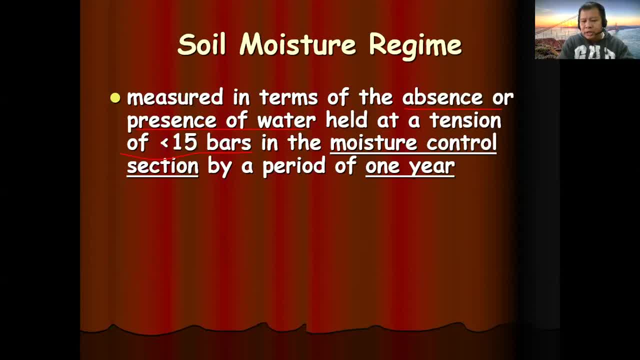 absorb water. plants can absorb water from the soil surface if it is healed by less than 15 bars. So more than 15 bars cannot be absorbed by the plants anymore. It's beyond their capacity to absorb water. So ang water greater than 15 bars dilit na magamit. So waters healed beyond 15 bars, maybe that? 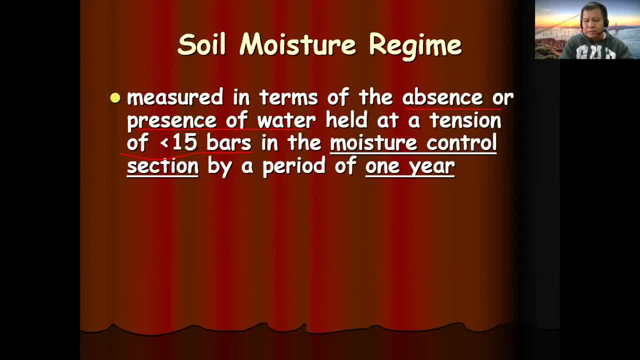 particular, soil is dry, Although there are some waters in there, that the water cannot be absorbed by the plants because it's strongly healed to the surface of the soil. Again, soil moisture regime: be sure, in terms of the absence or presence of water healed at the tensions of 15 bars in the moisture control. 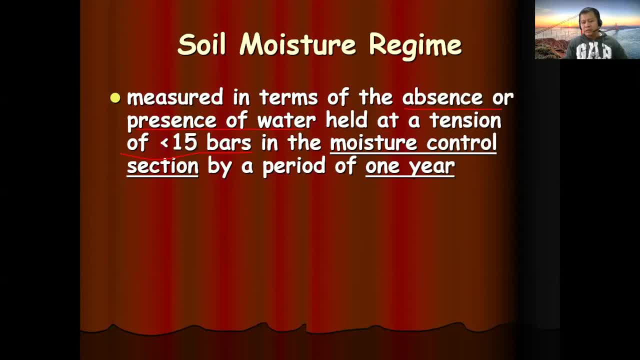 section by a period of one year. So I take note for that. Okay, the soil control section. So, unlike the soil temperature region, the soil control sections of the soil temperature region is 0 to 50 centimeter, But soil moisture region the control section is varies according to. 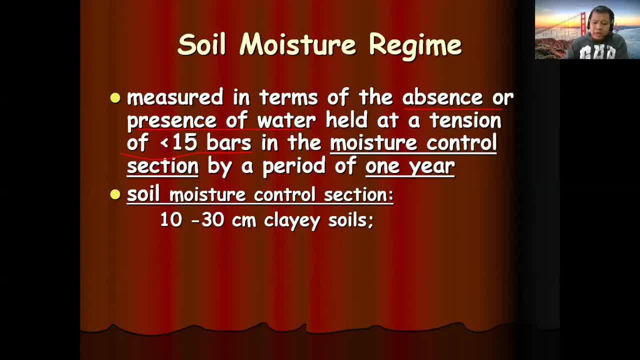 different types or different types of soils, For example, soil moisture. moisture control section for soil moisture regime of clayey soils: if the clayey soils, the control section should be within 30 centimeter. up down to 10 centimeter for clayey soils. 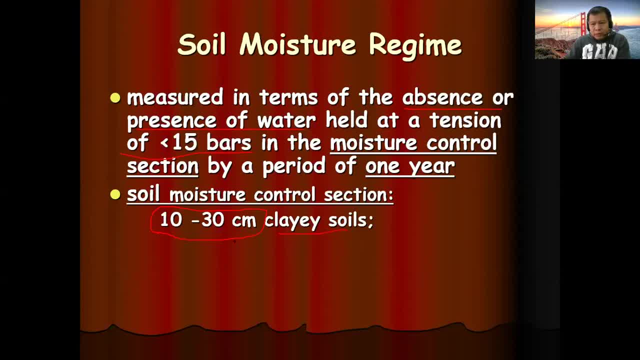 So why is this? so Because the clayey will hold waters longer than compared to sandy and salty soils. So this is the control section of moisture in clayey soils. What about in loamy soils? So the control sections for soil moisture regime for loamy soils is within. 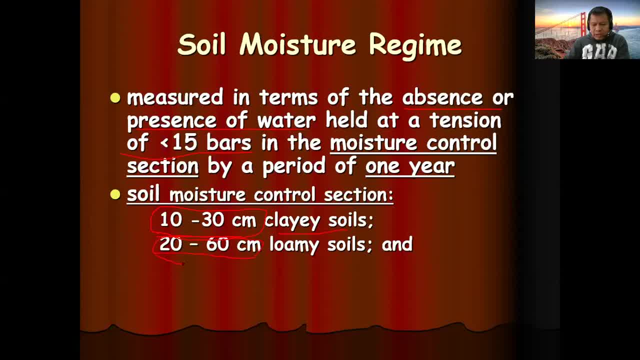 20 to 60 centimeters depth. Okay For loamy soils And for sandy soils. so we are to consider a depth of soil control section for moisture regime from 30 to 90 centimeters. Why is this so? Because water. 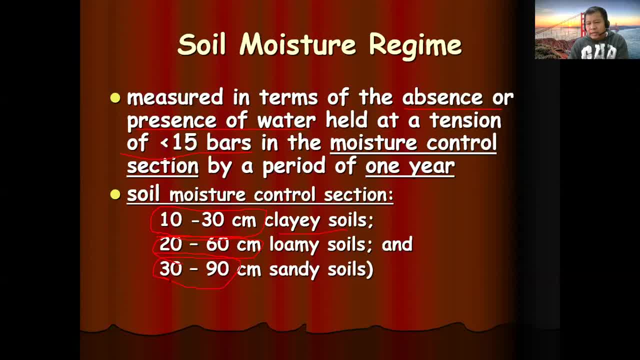 in sandy soils would easily drain and percolate downwards. That's why you have to. you know you have to, so. But the point is the soil moisture control sections varies according to the different types of soil texture, because clayey, loamy soils and sandy soils salty. 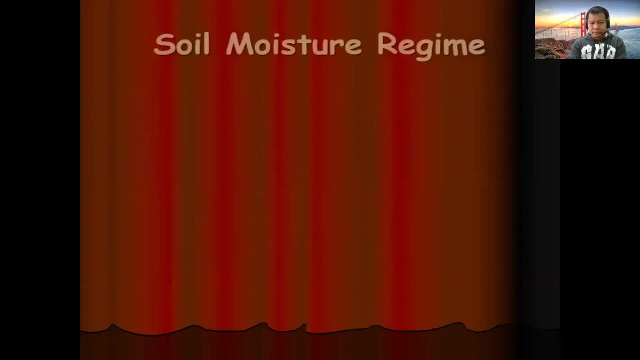 soils. these are soil textures, So take note for that. So what are those different soil moisture region? So we have the aquic moisture region. The word aquic or aqua. we're talking about water, Okay, what is this? So aquic moisture region: soil is saturated. 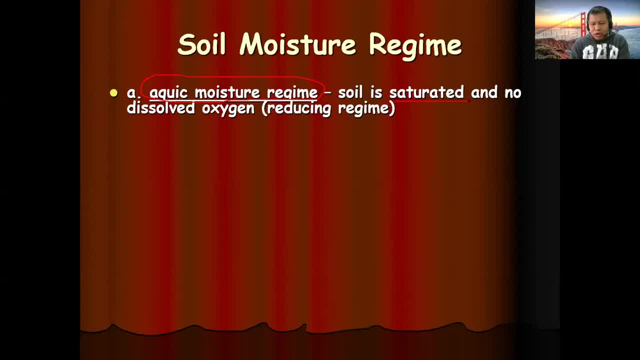 the pore space or the spaces. the pore space of the soils has been completely filled up of water, So I mean to say the soil is saturated and no dissolved oxygen. This is the reducing region, meaning to say no oxygen, So no dissolved oxygen. 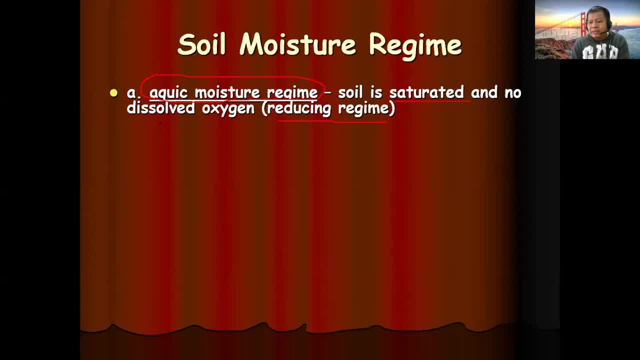 Katuladang. for example, if we have an empty bottle, if we have an empty bottle, if that empty bottle has no water, Therefore it is completely filled with oxygen or air inside in it. But if that bottle of water is completely filled with water, then there is no Air in it. So 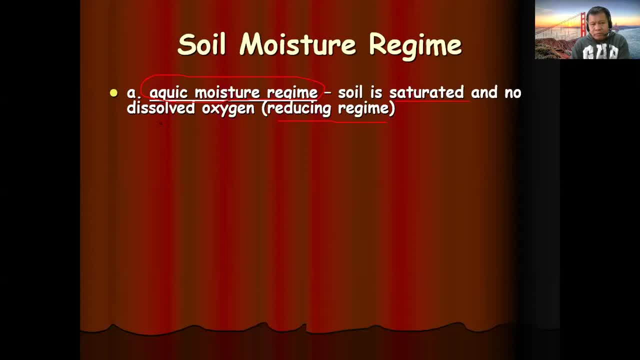 the relationship between water and air. if there is a full of air, then there must be no water. And Okay, You don't have water. Thanks, man. Okay, water will be filled in it. then the, the air has to displace outside thereby. 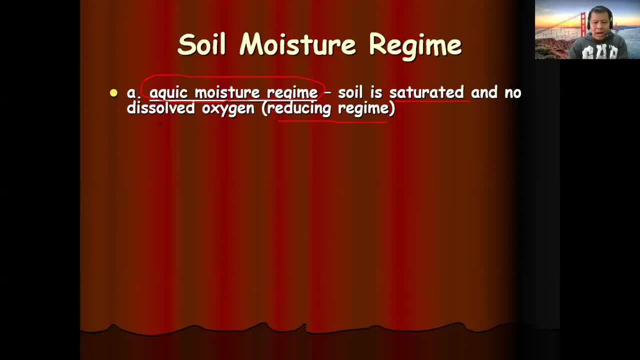 filling the bottle with full of water. so a quick moisture regime saturated me to say Puno, Puno, so too big at on utah, no, okay. so these waters are of submerged swells, connoisseur, Malia, nothing so far. the areas of a second, so another. 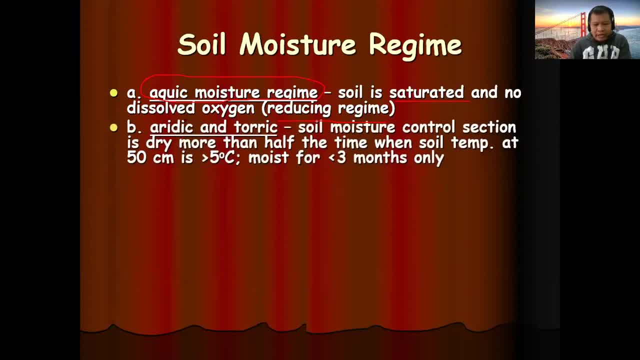 moisture region. we have a Riddick and Torik so I really can't work. so what is this? so almost your control sections is dry, dry. this is dry so much. your control section is dry more than half of the time when soil temperature at the 50 centimeter is. 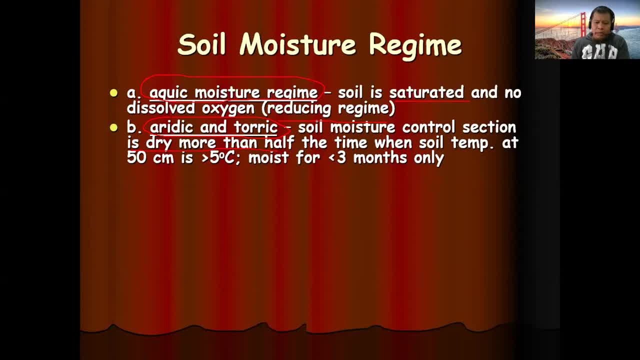 less than five degrees Celsius. moist for less than three months only. so moist for less than three months only, and the rest are dry periods. so think that for that, so I guess we have to change our the color of our printer, because- but I'm a contrast, as I know- I guess yellow is good, all right. so now, there we have the. 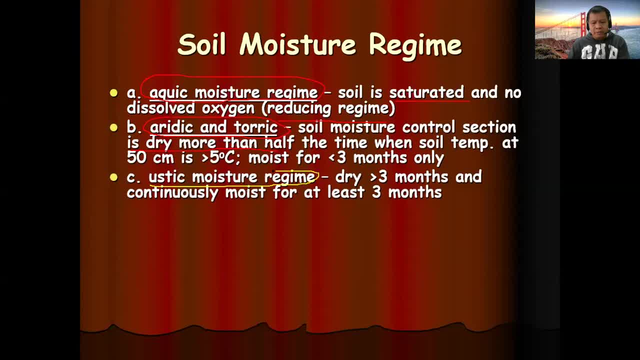 austic moisture region. okay, what is this? this I'll stick dry more than three months. okay, this will dry more than three months and continuously moist, or at least three months. so dry for more than three months, then moist for at least three months. so con basa mancia, anglopi supine kamata搂. 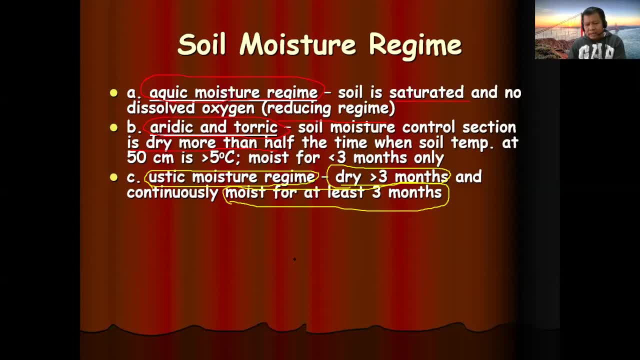 boss prayer and 3-mons, but and ripe or unit is more than three months. so this is is the austric moisture region. so ito, yung mga lupa sa mga sa mga maiinit na lugar. okay, another: we have the odic moisture region. so what is the odic? 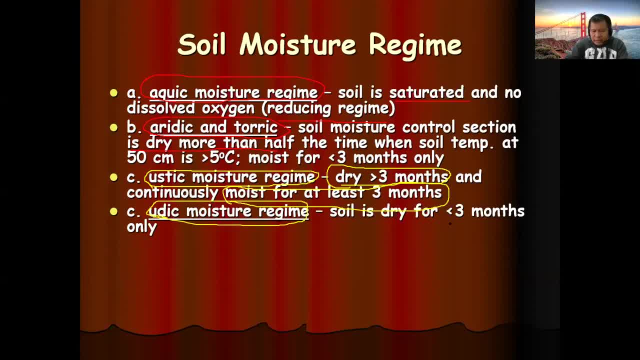 moisture region. so sewage dry for less than three months only. so less than three months only. this odic- look at the uh spilling odic moisture region- dry for less than three months only, okay. another moisture region: we have the ciric. you have the ciric moisture region. so what is this? 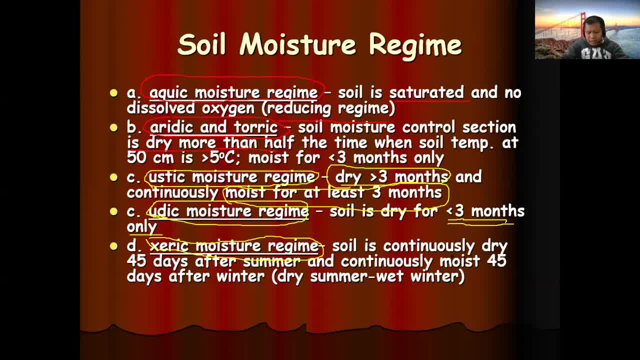 ciric is continuously dry 45 days after summer. so after summer, 45 days of the summer, dry parents here and continuous waste 45 days after winter. so this was is dry after summer and wait after winter. so 45 days after summer, dry, then 45 days after winter, moist. 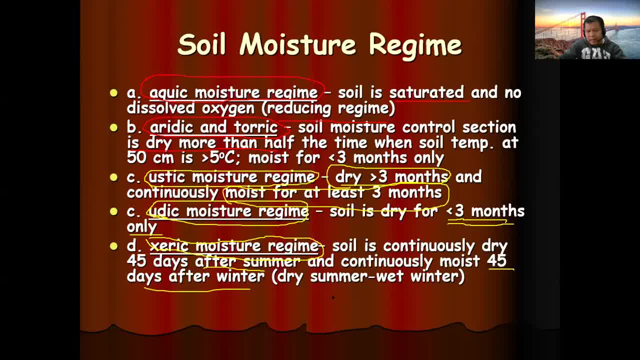 so these are belongs to acidic moisture region. okay, don't look for that again. the same with the soil temperature region. you have to develop your own acronym in here, uh, to aid your uh memorization. okay, then you can share your uh acronym. then you can decode later on. so 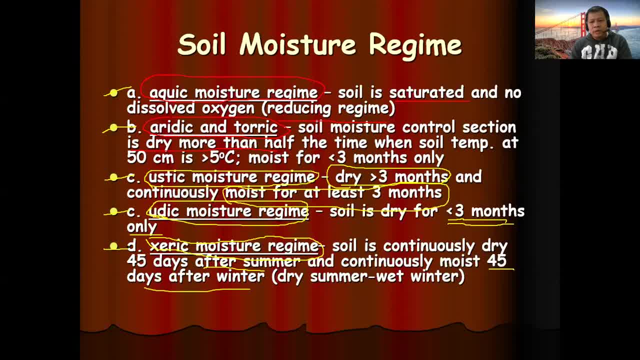 uh, i suggest that, uh, for a group. uh, we must have a uniform, um acronym for this, to aid or easily recall and memory. okay, so try to do that. we have a quick aridic. we have austic odic dick silly. well, I put like the one, two, three, four and five. so come here up on. 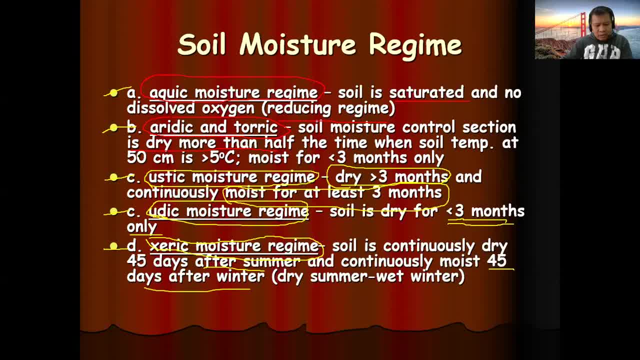 kayoga Moana, acronym. little song going along. memorize the first one, then the last one, then then I was a guitar memorize. try to develop your own technique for memorization that you can recall a silly later on. okay, so that's it. so you know, we have so well that. 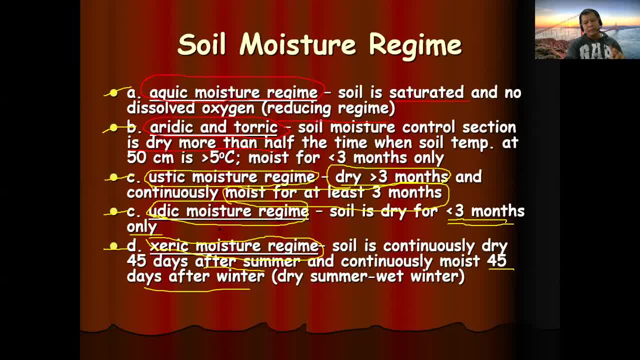 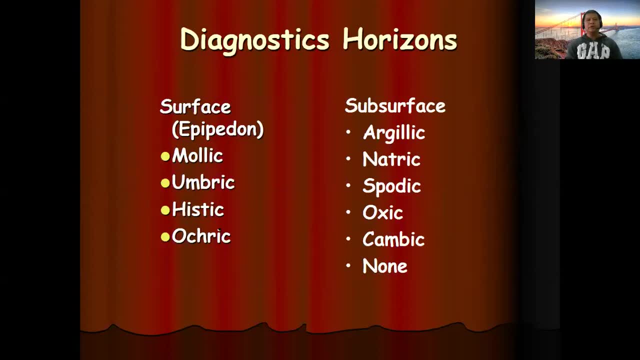 temperature region and we have this will moisture region and take note the control section for the moisture region which bar is with the control sections for that temperature region. okay, control section virus. so another important characteristics to be studied when we are to classify soils is the diagnostic horizons, diagnostic. 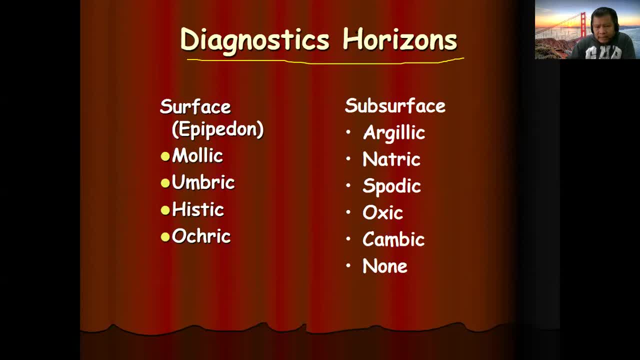 horizons. I know you my run or Makita, not inside horizons, and you might answer a horizon and you might answer B horizon. okay, so there's some say, there's some examples in here. you have the diagnostic subsurface horizon or the epipedon example of that. we have the mollick on brick, he stick and okra, but what are? 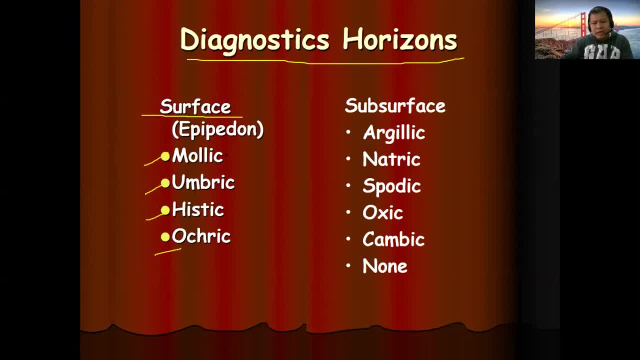 those. no, these are the basic features. these are the basic features that we can observe of this. anything on lands in the same pond for the study to do, the more shaped Z na yung makikita natin doon sa subsurface, maybe on a, B? 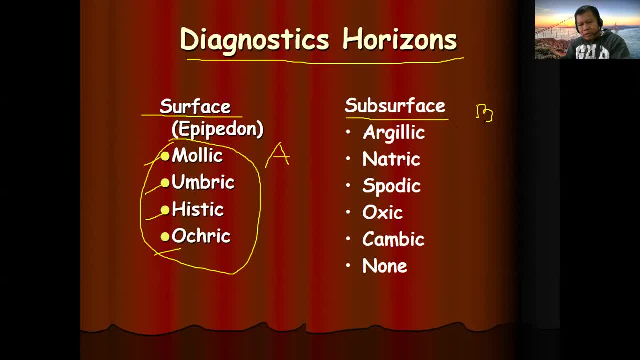 and part of a C horizon. no, Ano yung mayroon doon sa mga makita natin, sa mga horizon na yun subsurface, So posibleng may makita tayo doon mga argillic. 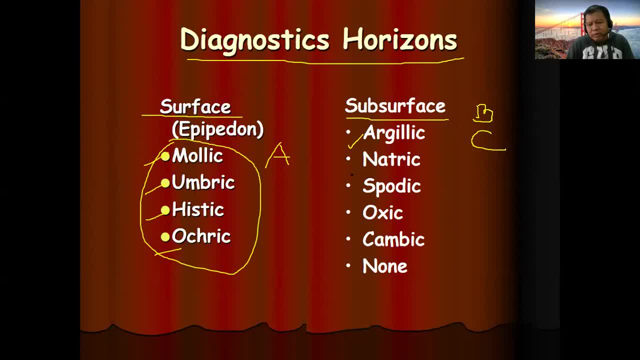 subsurface diagnostic horizon. Maybe mayroon tayong natric as a short understanding. Argillic is more on clays, Natric is more on pseudome Sputic- maraming mga accumulation ng sputic doon. 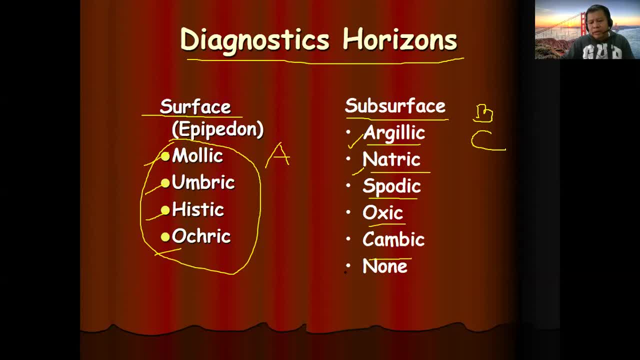 Oxic is oxides, Scambic is lime Minsan. mayroon tayong subsurface diagnostic horizon na wala tayong makikita. no, This is just among the examples of the diagnostic subsurface horizons that can be observed. 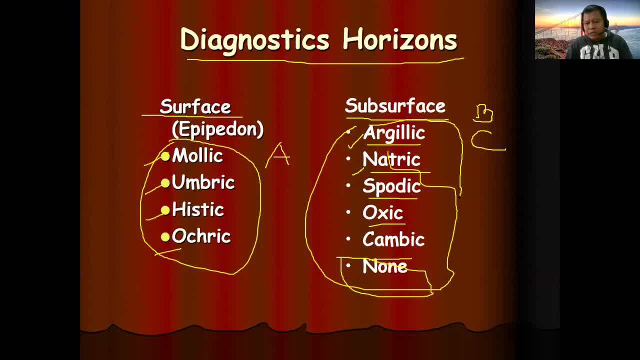 in the diagnostic subsurface horizon. But marami pa mga examples. These are just a few. no, Okay, So itong mga argillic natric, sputic, oxic scambic, talagang hindi, natin ito makikita. 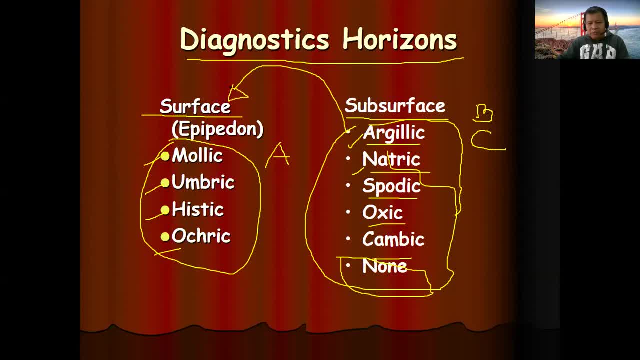 sa surface or epipedons. Di na ito makita Ganun din ito ding mga subsurface epipedons, itong mollic, ombric, histic and oculic- is cannot be observed in the surface horizon. 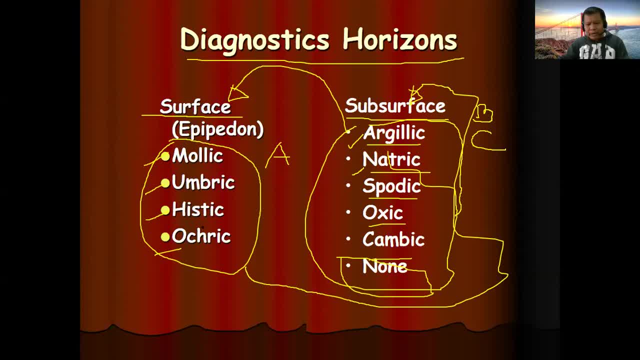 So di na ito makita ang epipedon kaling mollic ombric and histic. di na ito makita sa subsurface Ikinibong argillic natric sputic oxic. 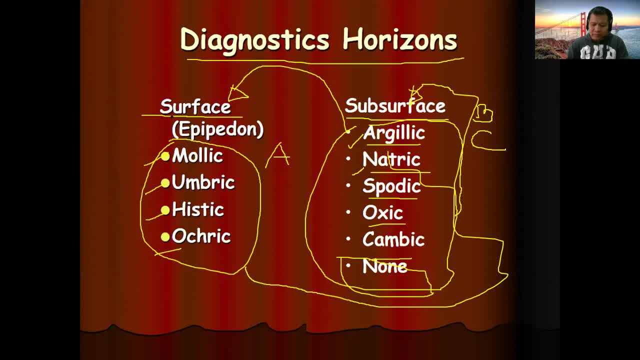 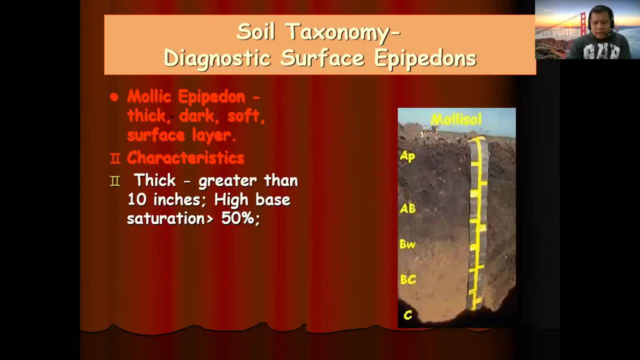 and scambic di na ito makita sa surface horizon. Okay, But what are those? What are those? Well, first, okay, So we have example in here. So we have, for example, soil taxonomy. 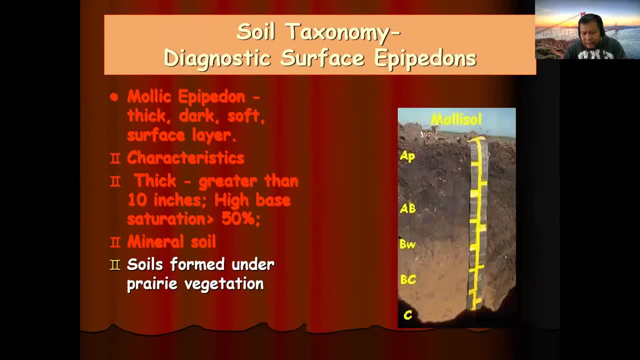 So diagnostic subsurface horizon, So ano yung makikita natin? I would like to emphasize the the subsurface horizon. So kung tignan niyo ha, sundan niyo itong. itong aking cursor. 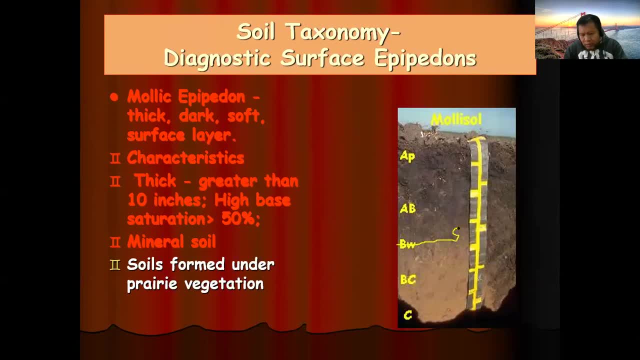 So iba yung kulay sa taas. kumpara dito sa sorry, kumpara dito sa baba. This one is the surface or the A horizon. Mayrong mollic, mayrong mollic na epipedons. 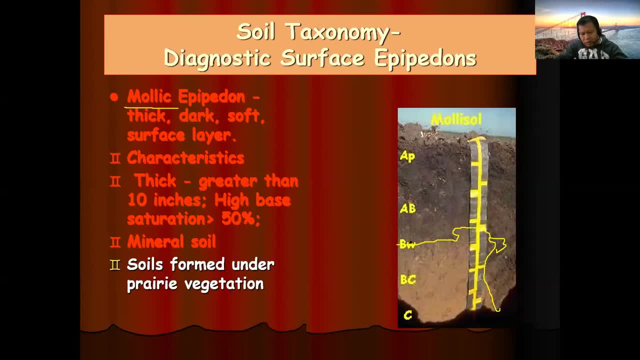 So itong A horizon, we can observe na, although mayrong diffuse ng A of B, so makikita natin, is mayrong mollic epipedon dito. What is mollic epipedon? It is a thick, dark. 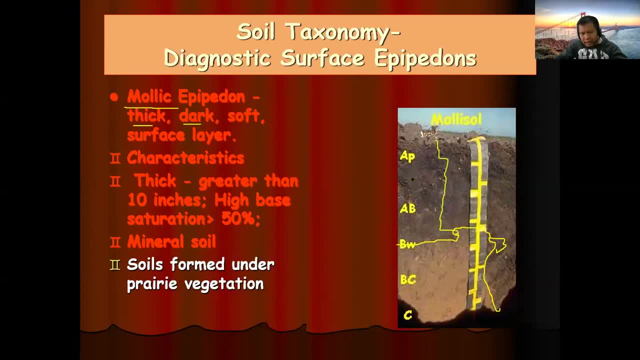 So this is a thick baga siya. no, Thick and dark, Dark color compared to the color below. So mas darker ang taas, lighter ang sa baba. So this is a thick, dark, thick, kasi medyo. 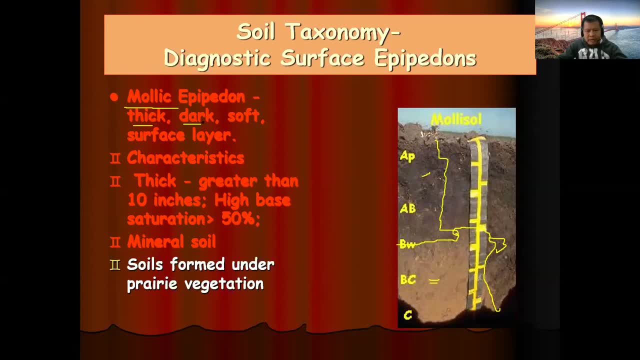 medyo malapad siya So thick, dark, soft. And this portion is medyo less dense, Less compact, Humog siya Hindi siya matigas Okay, Soft surface layer. So this is thick, dark, soft surface layer. 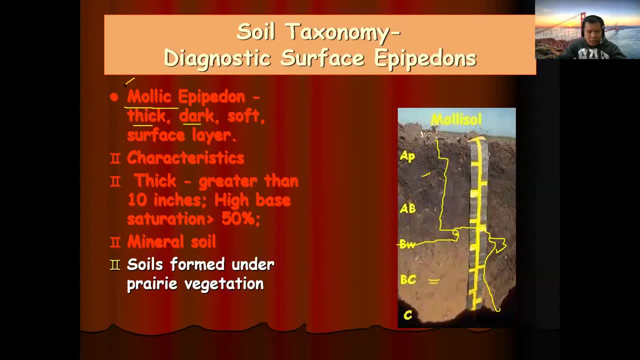 found in A horizon. Therefore, it's considered as a mollic epipedon. Now, knowing of the different diagnostic features in the diagnostic horizon would help us to classify swills based on their swill order. okay, And this particular example. 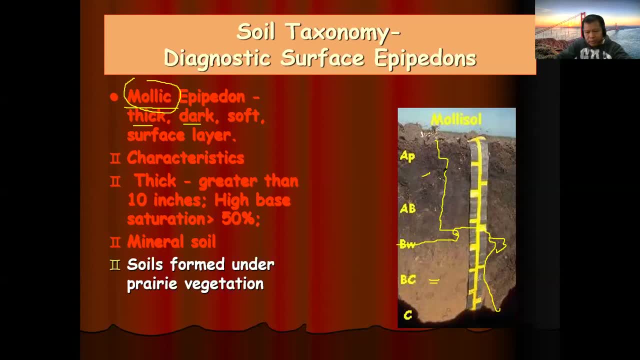 if we can observe a mollic epipedon in a surface diagnostic horizon, eventually that swills belong to a swill order of mollisol Again. so the distinguishing feature of the swill order mollisol is a mollic epipedon. 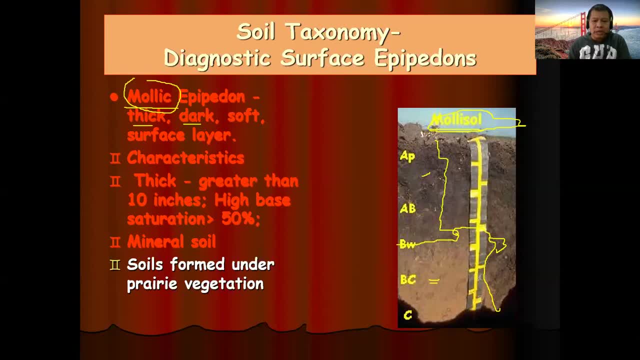 So whenever we can observe a mollic epipedon in an A horizon, then eventually we will. you know, we would classify that swills belongs to a swill order mollisol. So kasi mayroon ding mga swill order no. 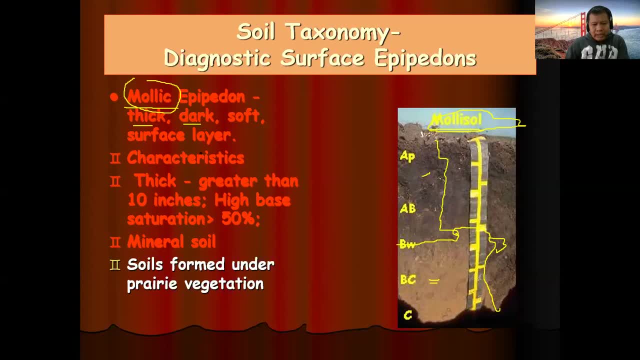 Later on. Discuss natin yan later on. So ano yung characteristic ng mollic epipedon? Yes, sinabi doon thick, Ang thickness niya is greater than 10 inches, So this one probably this. 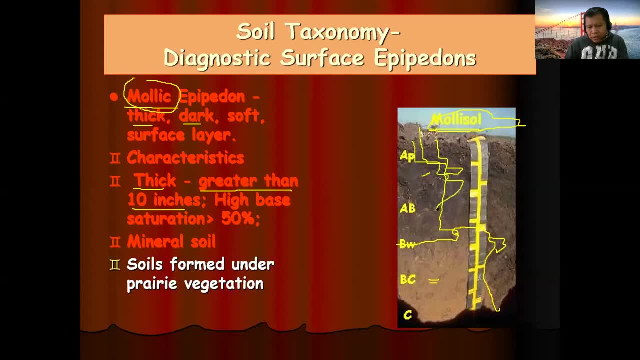 this portion is greater than 10 inches. Okay, And another characteristic niya is high base saturation. Pag sinabing base as opposed to it and contrary to acidic, so basic and acidic, So high base saturation. High base saturation of more than 50%. 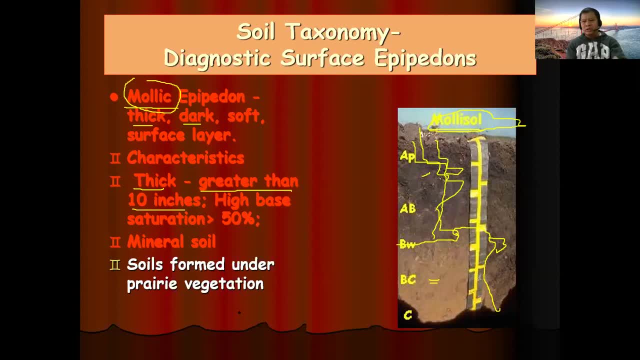 Pag sinabing mga base, we're talking about cations, mga basic cations or alkaline cations. So we're talking about calcium, magnesium, potassium, ammonium or any basic or alkaline cations for that matter. 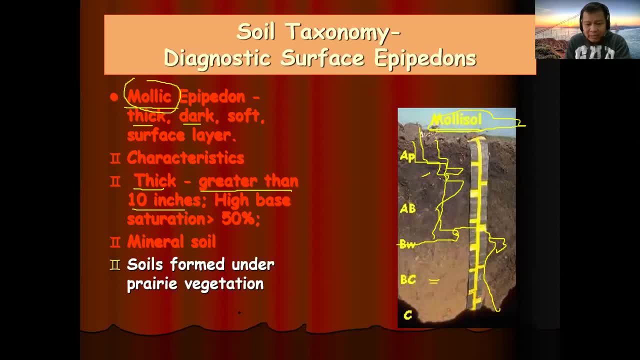 So okay, maraming mga base diyan, So hindi siya acidic, kasi maraming siyang base na more than 50% ang base saturation niya. On the other side, mas gamay yang acidic cation saturation. 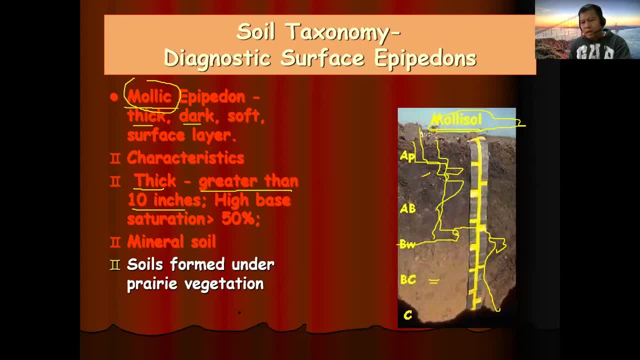 So maraming base diyan, Maraming calcium, magnesium, potassium. Ano yung mga basic cations na mayroon diyan Marami doon. So gamay lang diya Ang aluminum, gamay rin po din ha ang iron. 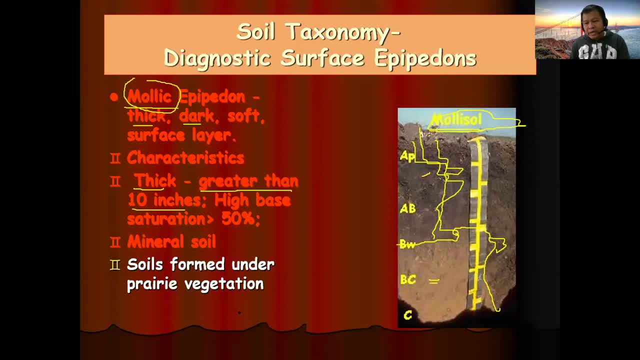 o hydrogen, Kaya mga acidic mo ng hydrogen, iron and aluminum. So wala kayo sila sa mollic epipedon, Kaya mostly basic cations ang mayroon diyan Okay, And of course the mollic epipedon. 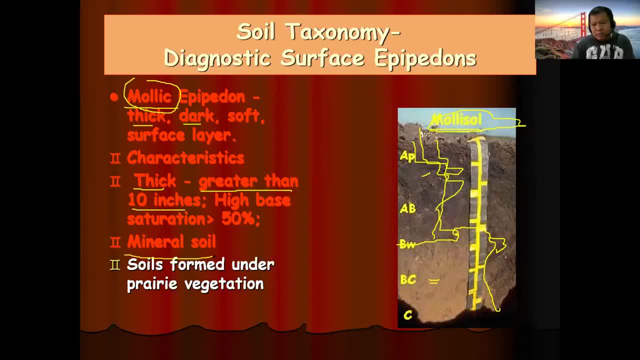 is a mineral horizon. Anong ibig sabihin ng mineral horizon? It is a mineral horizon because this mollic epipedon is derived from rocks and minerals. So therefore, when it is derived from rocks and minerals, their parent materials is. 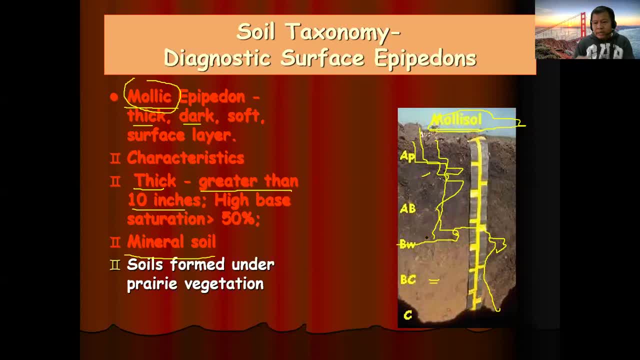 rocks and it is considered as a mineral horizon. If the parent materials belongs to an organic source, it would not be considered as a mineral source, It would be considered as organic soils. So take note po dat, And usually itong mga. 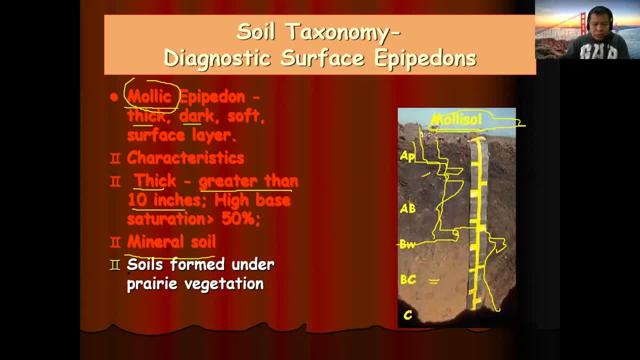 mollic epipedons or mollisos, soils form under the prairie vegetation. Pag sinabi yung mga prairie vegetation, we're talking about the grasslands, May mga damuhan dati. Okay Ganun, So take note po dat. 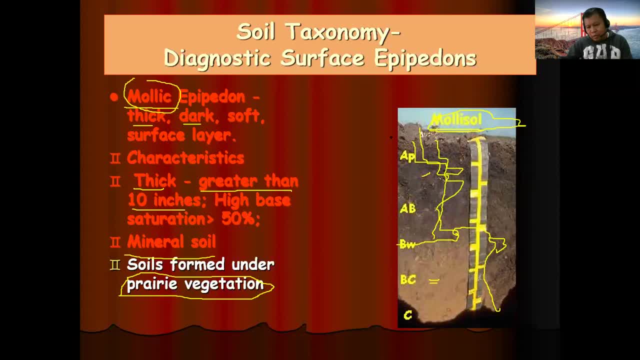 This is the e-horizon. the darker portion Mayroong mollic epipedon din mollisol Sa baba is the subsurface. So we cannot observe a mollic epipedon in a subsurface, Only in the upper. 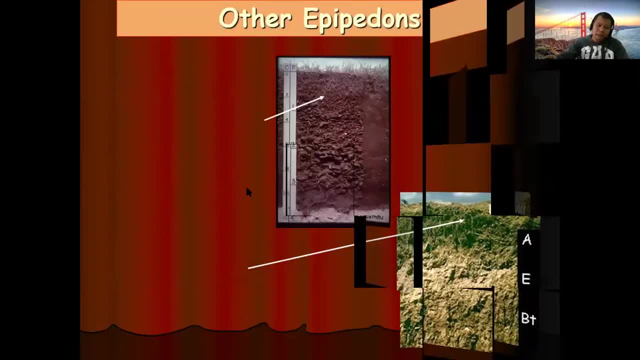 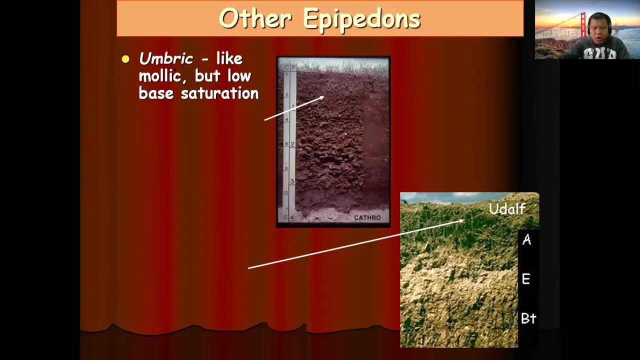 surface horizon. So another another diagram, another diagnostic surface horizon is the ombric Ombric. Okay, So ombric it is like mollic, but low base saturation. So in terms of dark thickness and softness, 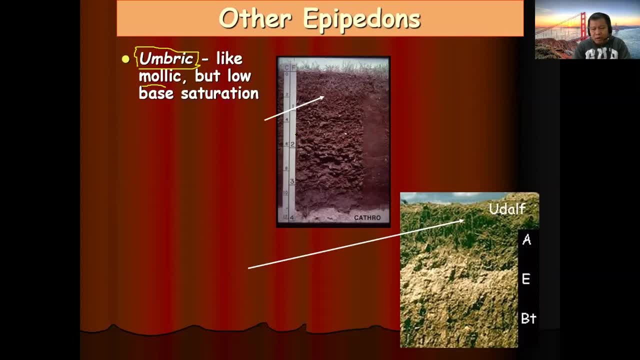 the same with the mollic, but what varies is the chemical composition, because, compared to mollic, it has now a low base saturation. If the mollic has a more than 50% base saturation, then ombric is definitely not more than 50%. 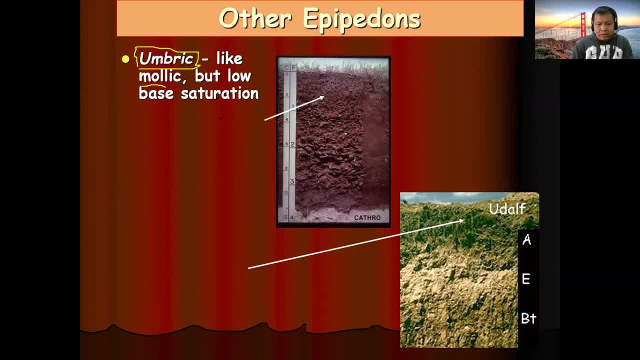 base saturation- Okay again, So take note. We also have a hystic Hystic from the word organic soils Saturated with water And more than 20%. This is 20%, So take note. 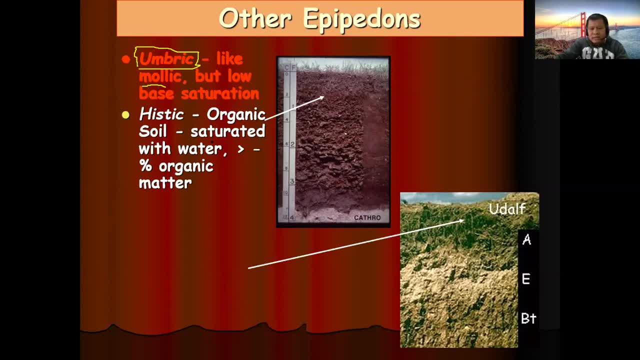 Hannah, Hystic from the word organic soils Saturated with water, And more than 20%. This is 20%. So take note, Hannah: 20% organic matter. So this is not a mineral horizon, because it is. 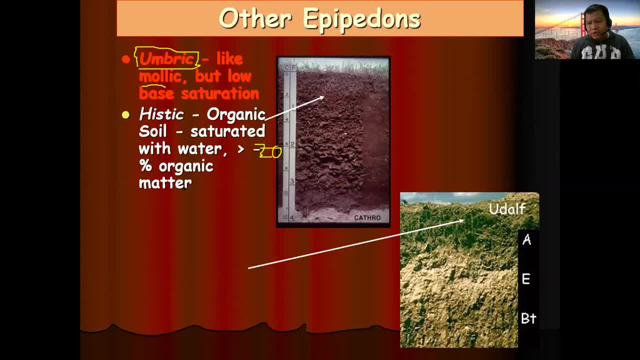 from organic source. So this is hystic Organic soils saturated with water, More than 20% organic matter. So that is organic matter. Okay, If you have to look at this layer, it is not that visible, But 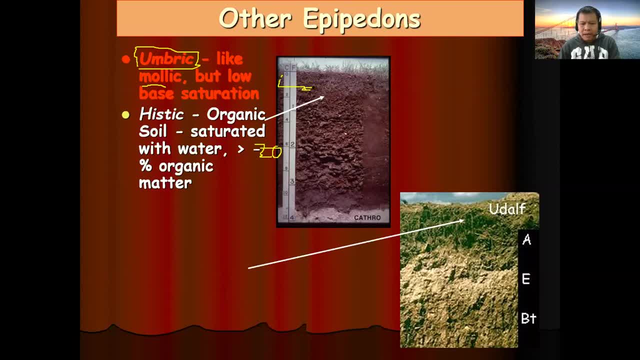 here because we are talking about hystic. there are some organic soils in here, As I would say humus, Decomposed or partially decomposed debris of plants. Maybe there are twigs or branches of grasses and any sorts. 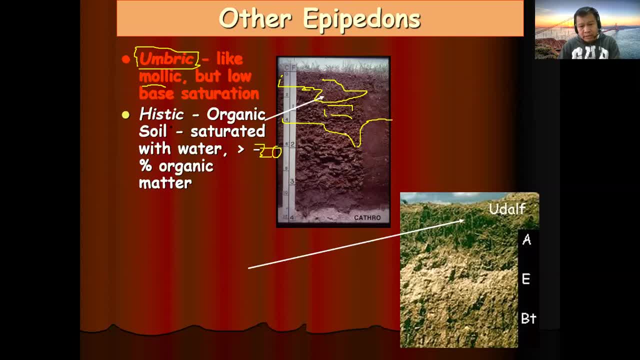 of plants or partially decomposed leaves- This is hystic- So saturated with water. So I mean to say this is submerged in water, because when organic matter is submerged in water it will decompose, It will remain as tissues or partially. 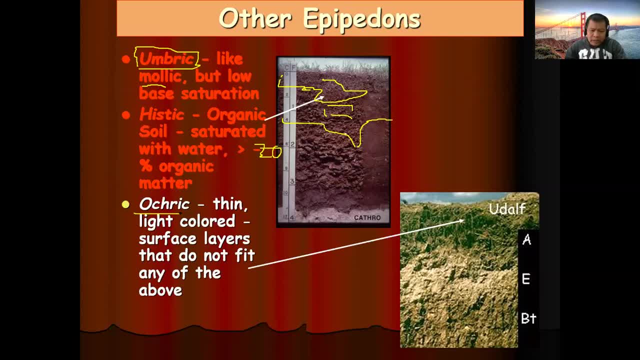 decomposed tissues. Okay, So another example. It is a thin. Look at this one. Okay, This is a portion of it. Okay, This is thin, light colored surface layers that do not fit to any of the soil. The 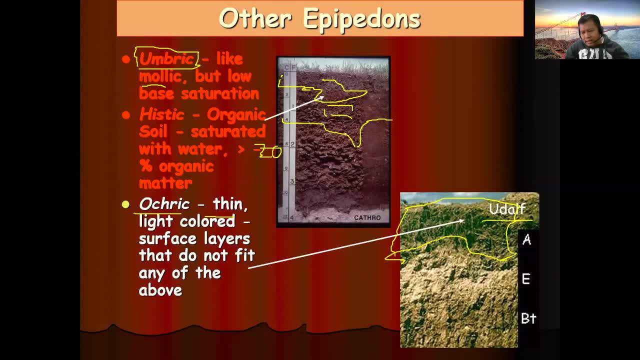 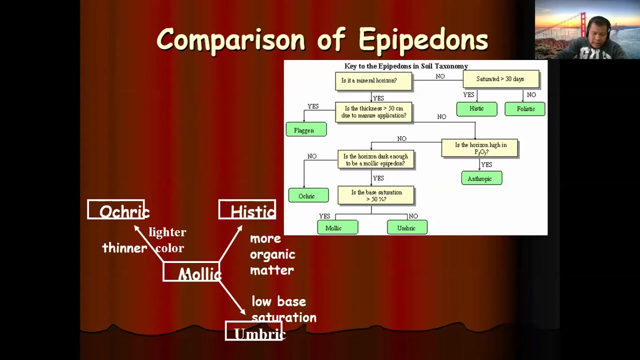 name of the swells we have the udalp, So the soil moisture region is udic and belong to the order alfisol. So we have to deal that clearly. on thick, dark and soft: more than 50% base saturation. 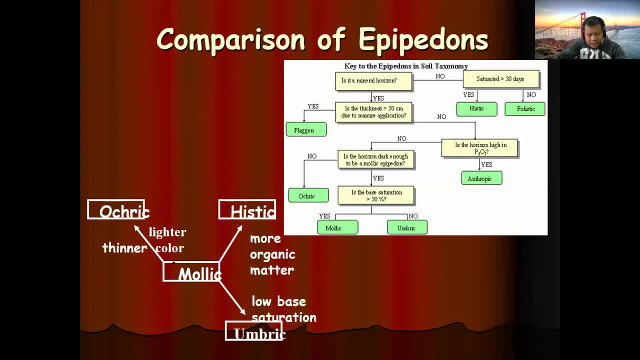 Compared to mollic, if it is lighter in color and thinner in the surface of organic matter, then that must be ocric. Compared to mollic if it has more than 20% organic matter, then that must be histic. But compared to mollic if it has a low base saturation. 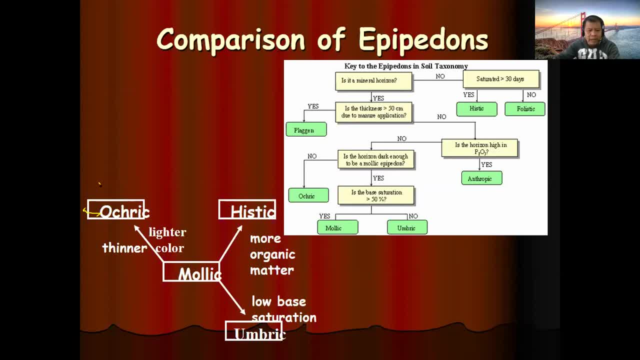 it must be unbric. So this is how we memorize, how we understand, so that we can easily understand the different surface diagnostic horizon and a-horizon. I also included in here the key to epibedons in sweet taxonomino so that if we are to classify swales, 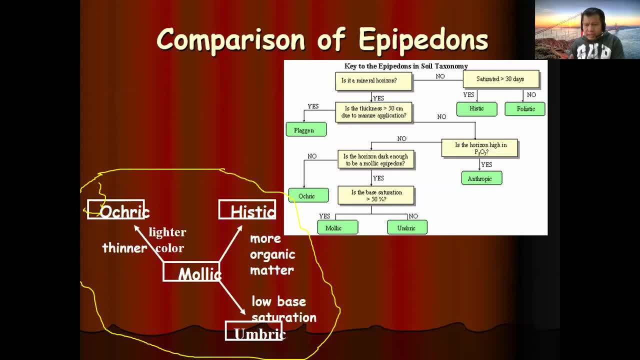 based on swale order and diagnostic horizon. so is it a mineral swales? If it is a mineral swale, then it has the thickness of more than 50 centimeter in the epibedons due to manure application, If it's having manure application. 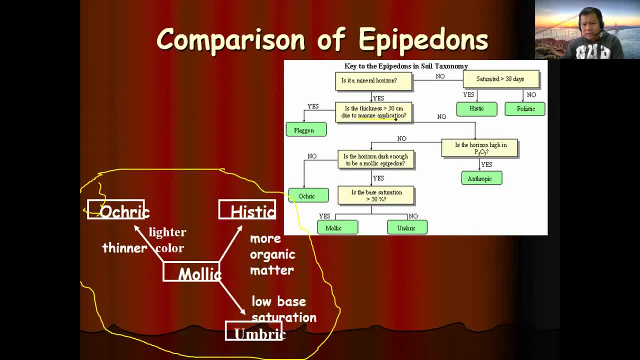 I am abuno because of the human action. If it has a thickness of more than 50 centimeter due to a manure, yes, then that must be called as aplagin diagnostic horizon. The thickness is more than 50% due to manure application. 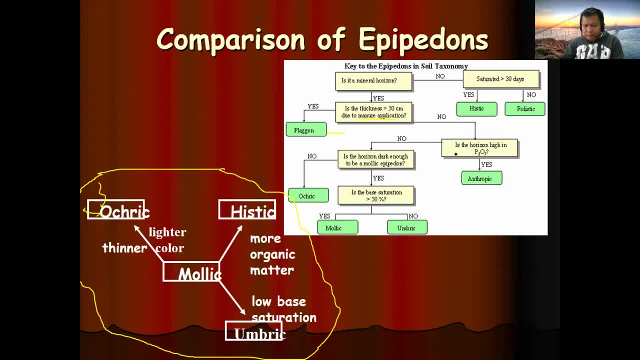 No, if the horizon is high in P2O5 or a posporous, if it is more than posporous because of human application to the field, then it must be an anthropic. Anthropic. now is the accumulations of posporous. 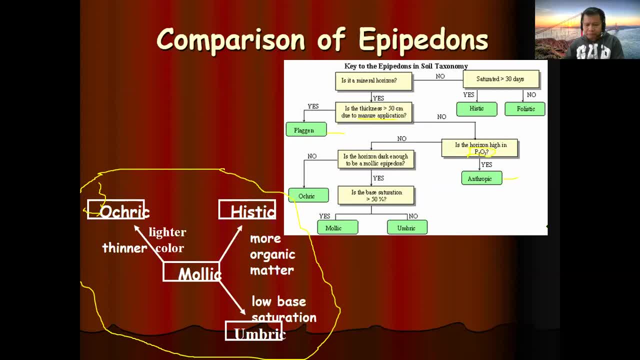 in the a-horizon anthropic horizon. So that's how to analyze: Is the horizons high in P2O5? No, Is the horizon dark enough to be a mulic Con? darksia is the base. saturation more than 50%. 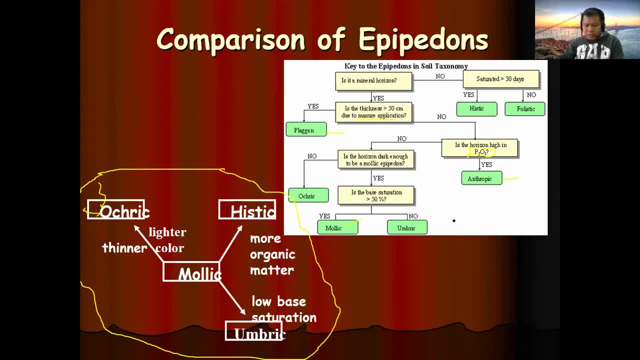 Then it must be a mulic. The base saturation is not more than 50%, then it must be an ombric. So, going back in here, is the horizon dark enough to be a mulic? con delicia dark, It must be an ocric, okay. 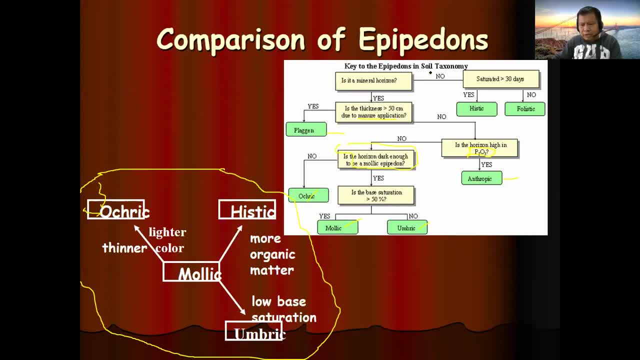 So, for example, it is the mineral horizon? No, it is not a mineral horizon. Is that saturated for 30 days? So submerged mulicia. so to be submerged for more than 30 days? Yes, if it is submerged, then it must be histic. 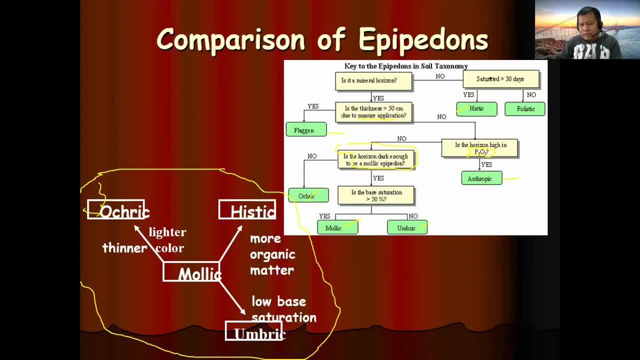 more than 20% organic matter Saturated for 30 days. No, it must be a holistic. So this is how we aid ourself in categorizing swales in a different diagnostic horizon. These are example of diagnostic horizon: plagine, histic, holistic anthropic ombric. 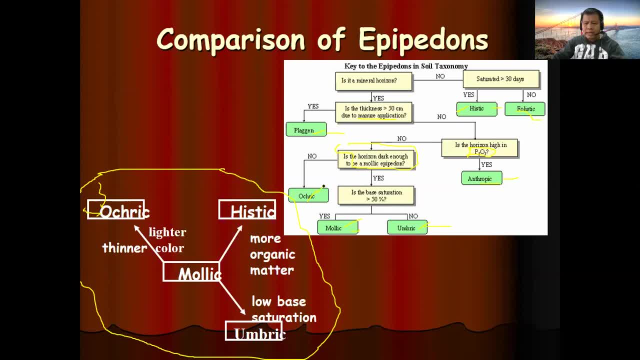 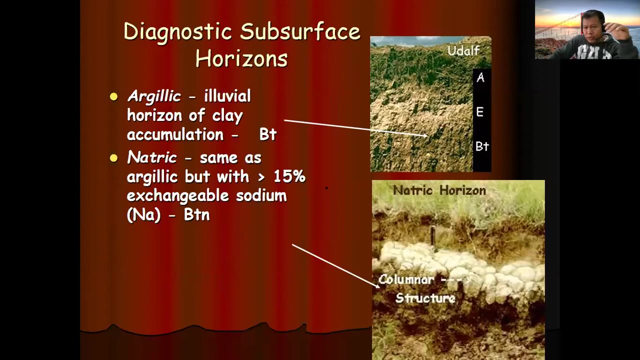 mulic and ocric. So try to understand this illustration, because this will help you in differentiating different diagnostic horizons compared to the other. Okay, let us proceed now. Now we also have the diagnostic subsurface horizon. The one we discussed a while ago is for a surface horizon. 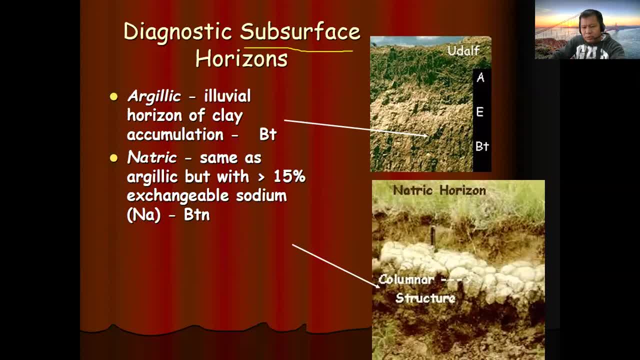 Now is for subsurface: Anything that we can observe in the B horizon and as well as in the C horizon. An example of the diagnostic subsurface horizon is the argillic. When we say argillic, we're talking about the alluvial. 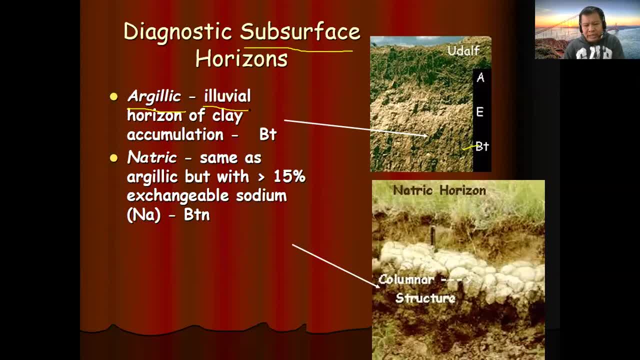 When we say alluvial double L, because there is an alluvial and a single L. alluvial deposition- another term deposition or accumulation. So when we say argillic, this is an alluvial horizon of clay. 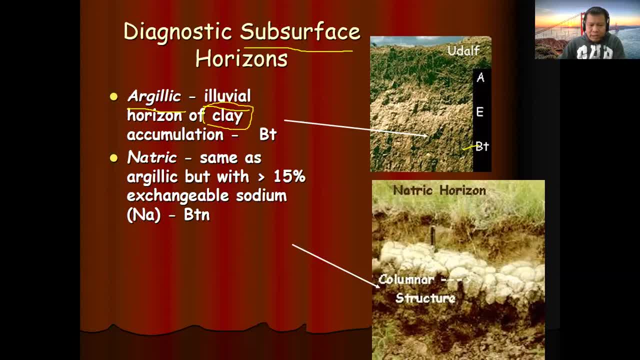 So there is a clay, but in argillic we're talking about argillans are clay. So we need to say there must be a clay deposition in the B or in C horizon. So, for example, this is the B horizon. 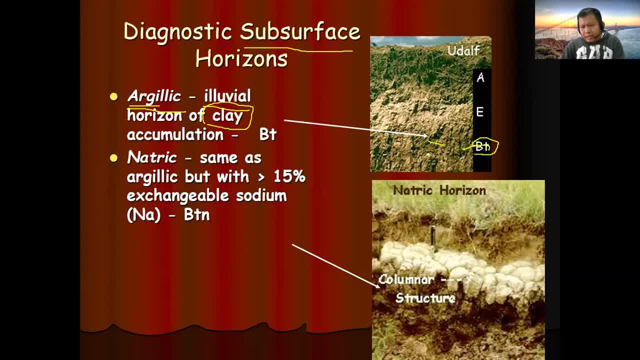 Bt is a connotation or presentations. Bt is refers to argillic horizon or the alluvial, or accumulation. So this is the accumulation of clay in the B horizon. So look at the Bt Whenever we see a Bt presentation in the horizon. 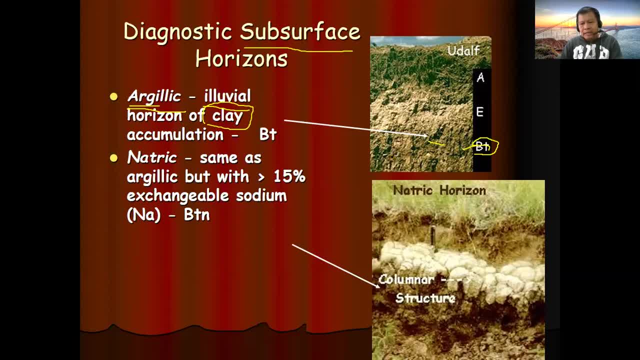 it talks about the accumulations of clay in the subsurface horizon. Okay, so another one. we have the natric subsurface horizon. So natric, this is the same as argillic. There is a clay, There is a clay accumulation in here. 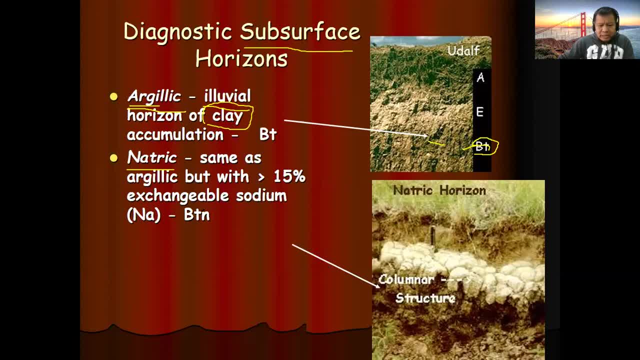 but with more than 15% exchangeable sodium. Okay, the same as argillic, but more sodium accumulation in this, in the natric, compared to the argillic. Okay, so in this example, so we have the natric accumulation. 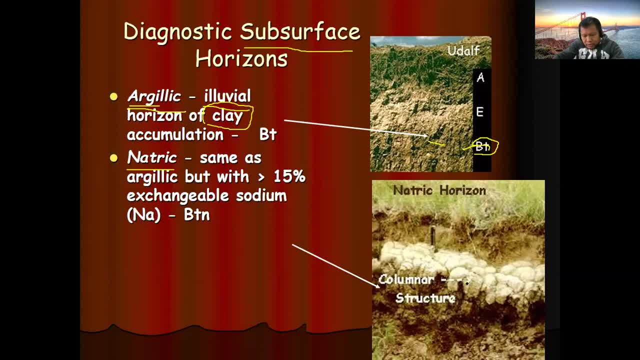 So natric accumulation in B horizon. and in B horizon there is a thing called there are columns, columnar structure, Columnar arrangement of soil particles. So in this columnar structure, for example, there is a column like that on the soil. 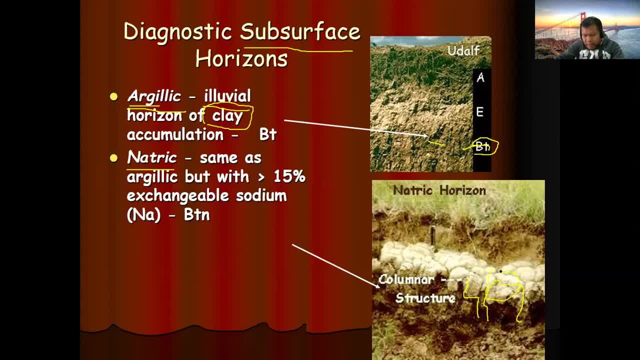 On the top there are white sodium cups. These are sodium right The sodium cups. the sodium cups on the column of the soil particle is because of the high amount of sodium in the soil. This is because of the high amount of sodium in the soil. 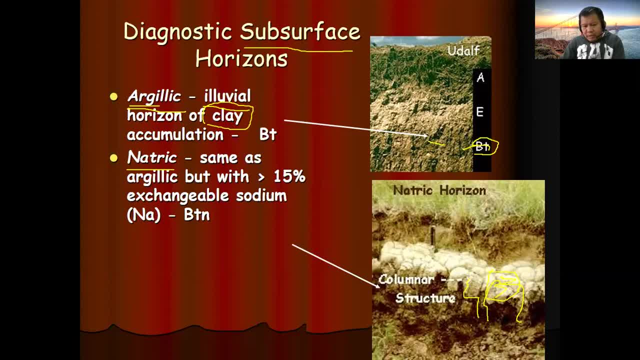 It is because of the high evaporation rate Particularly this. the natric subsurface horizons can be observed in the arid region, Saudi Arabia. because it is hot, so the evaporation is high, so thereby the water moves upward into the atmosphere. 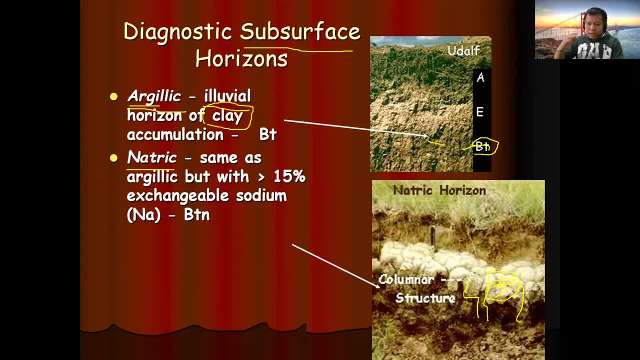 so the sodium that is brought by the water is left on the soil. when the water is raised, the water goes to the atmosphere, But the sodium? The sodium will not be brought to the atmosphere, so it will be left in the top columnar structure of the swales. 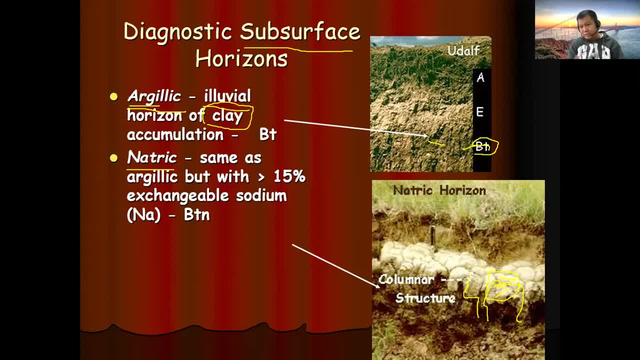 Later on we have to discuss the different structure of the swales and as well as texture, But this time we just be surprised with this discussion for the nitric. Well, nitric the same as clay accumulation in the subsurface horizon, but must have more than 15% exchangeable sodium in the surface. 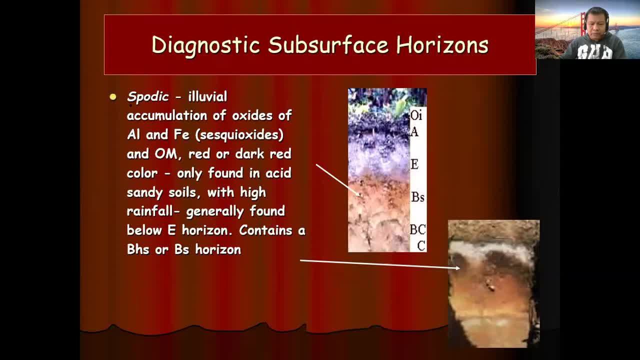 For example, we have the spodic. Spodic is the alluvial accumulation of oxides of aluminum and iron. This means that there is iron oxide, aluminum oxides, and these are called sesquioxides. Okay, Those again spodic: alluvial accumulations of oxides of iron and aluminum, or sesquioxides, and also organic matter. 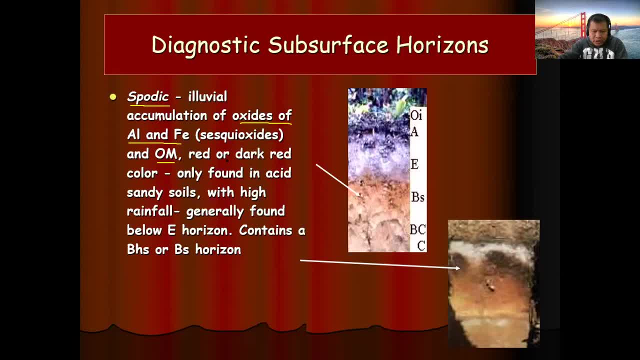 So alluvial accumulation of organic matter. This must be a red or dark red in color, only found in acid sandy swales with high rainfall, Generally found below E horizon. Contains a BSS or the BES horizon. Now, if you're looking at the BES horizon, 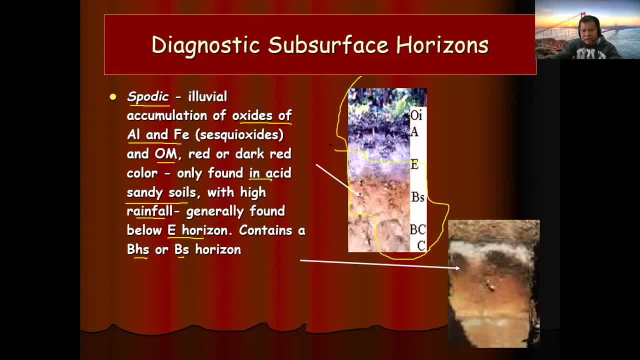 If you are to look at the layer of the swale profile, For example, the swale profile, Look at this one. I guess you have to change the order now, Anyway. So actually, an E horizon is lighter in color. no, 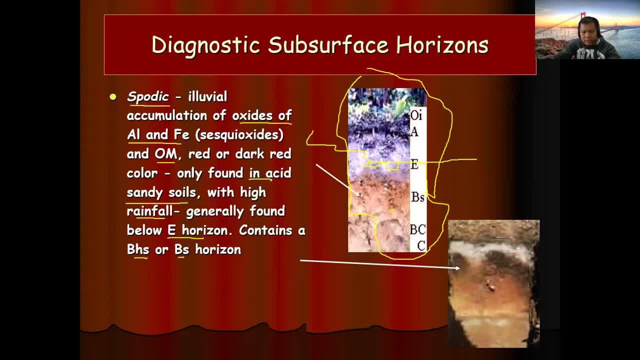 Compared to both below and above. Okay again, BES and BSS. So we have the BES in here, In this particular region. So the BES refers to a spodic, or the accumulation of oxides and aluminum oxides. 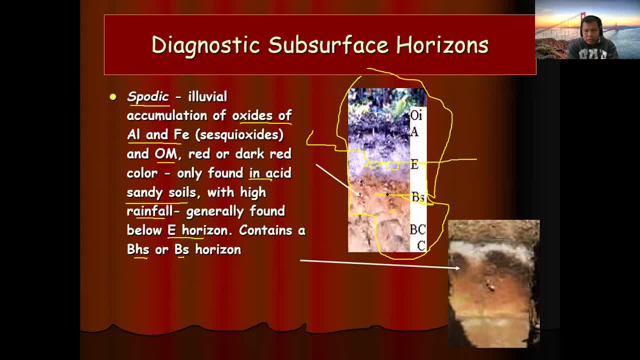 Usually swales with a spodic diagnostic subsurface horizons. This belongs to an old swales. The swales has been through a long period of withering Because, if you can recall, during our first topic, So the major and the final product of withering, 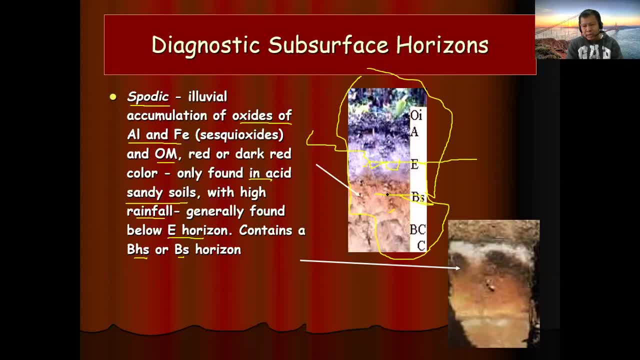 Is the oxides and hydroxides of aluminum and iron. So swales with a spodic categorically has less productive and less fertile swales Because they're acidic and old swales, Right. So another example we have of the diagnostic subsurface horizon. 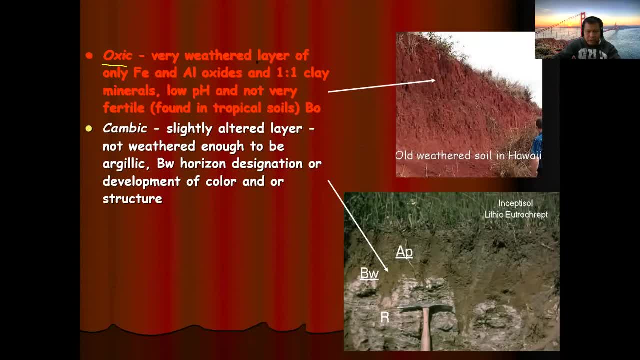 We have oxic Berry withered layer of iron, Of iron and aluminum oxides. Now, this soil that has oxic, This is older compared to the soil that has spodic, But these are old swales too. no, The oxics berry withered layer of iron and aluminum oxides. 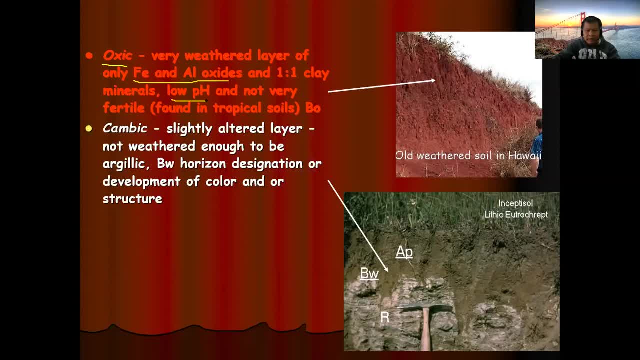 And 1 is to 1. clay minerals: Low in pH. These are acidic, Not very fertile, Because these are just figs Found in tropical swales And this is designated by BO In its soil profile. So in our example, 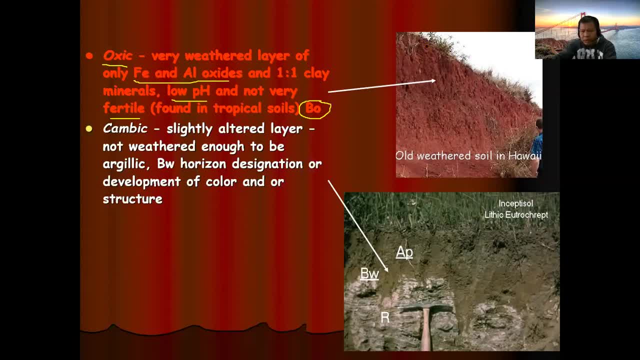 Look at this one Old withered swales in Hawaii, Although we can also observe swales in Philippines, In our province, Maybe in the oriental area We can see this. We can see this When we went up there in Hamigitan. 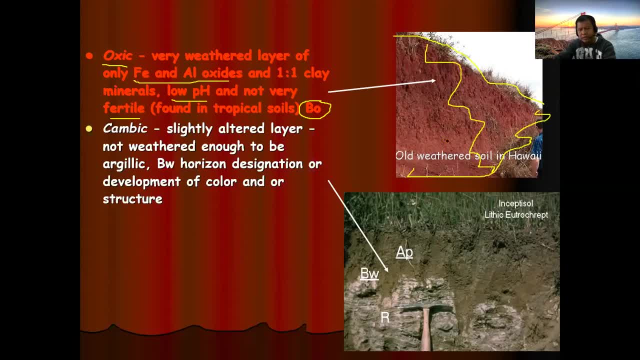 I saw this kind of soil- Okay, Really swales- So red Because it's an iron And These are acidic swales. no, So thank you for that, And Look at the thickness of the soil profile. 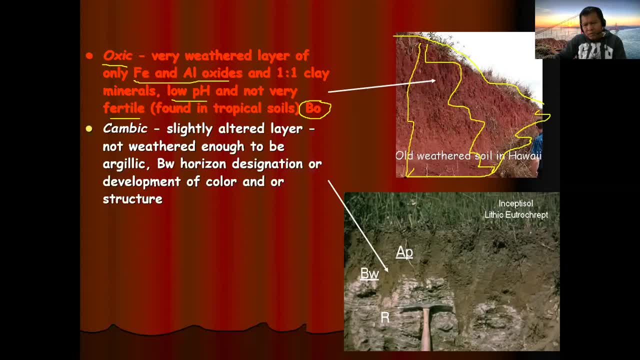 It's a bit thick. no, This is more than Maybe more than 150 centimeters, More than 1.5 meters- The layer of the swale, Because This has withered for a long time, So the soil has formed thick. 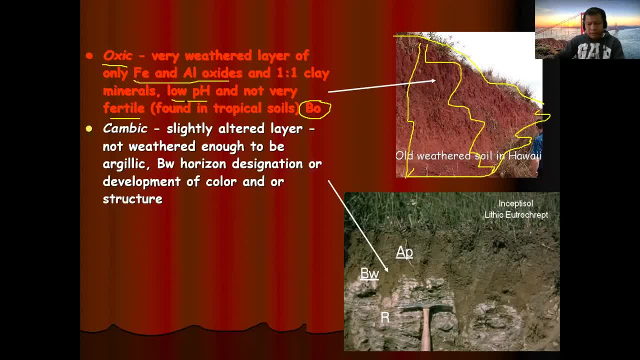 To a period of withering. So this is oxic? no So. another one that we can observe in the diagnostic subsurface horizon is the cambic. This is slightly altered layers Not withered enough to be argillic. 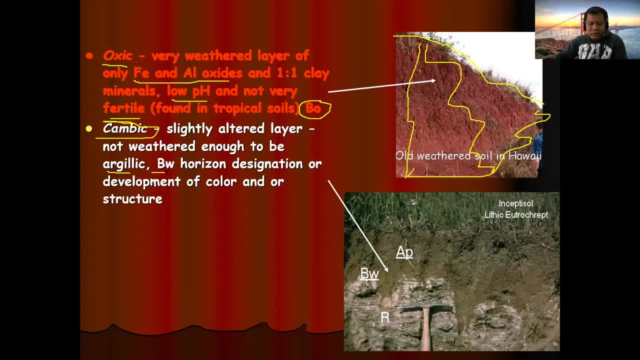 Glacial argillic Represented by BW in the horizon, Such as, for example, in this picture, Right B horizon. designations or development of color and or structure. So cambic, So cambic. usually is There's lime, no. 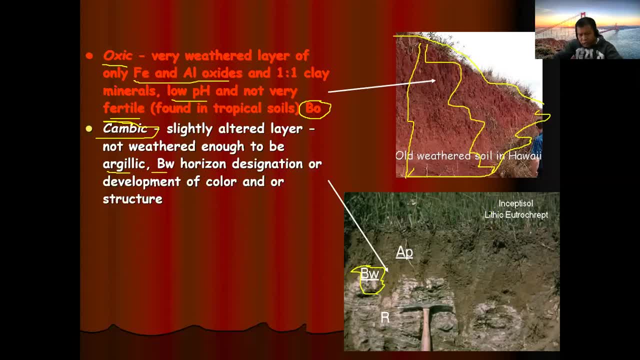 There's lime. An example: We have the swale name in here, Incepticol swales. This is called lithic utero crypt, So belong to incepticol order, The lithic utero crypt. Another example: In the horizon there's A horizon. 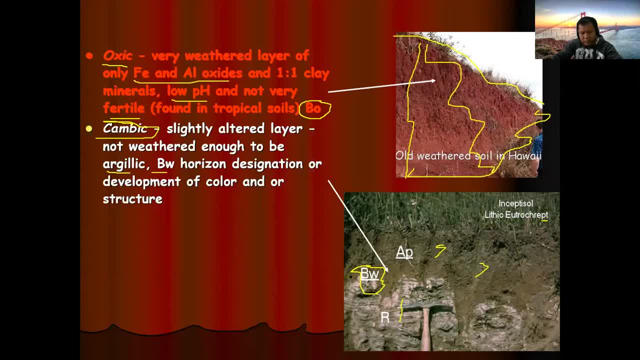 Down here there's B horizon. If you look at it It's not as old as the old swales, Because there's soil After that there's stones, Meaning to say the rocks has not been withered fully. Maybe this has been through a short period of withering. 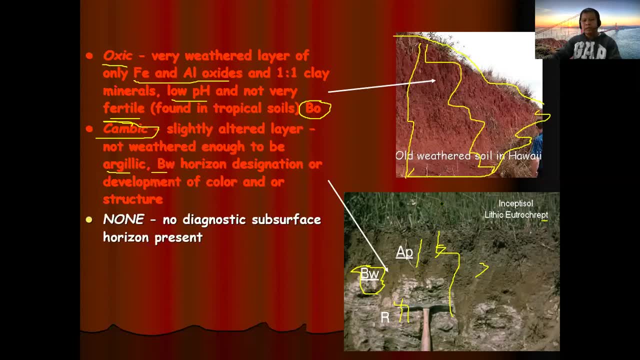 Like in this cambic Also, there are some instances that we cannot see any diagnostic subsurface horizon in the B or in C horizon. There are some different subsurface horizons, But for the purpose of this discussion So you have just to present a few of that. 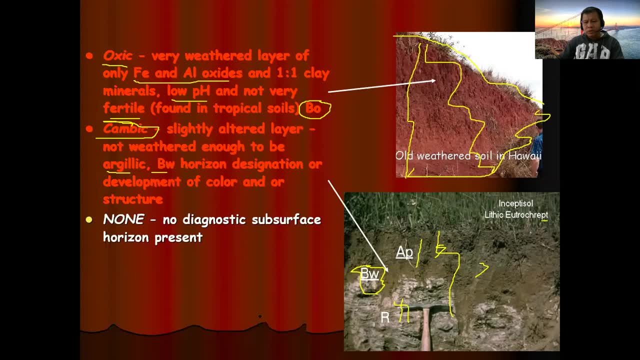 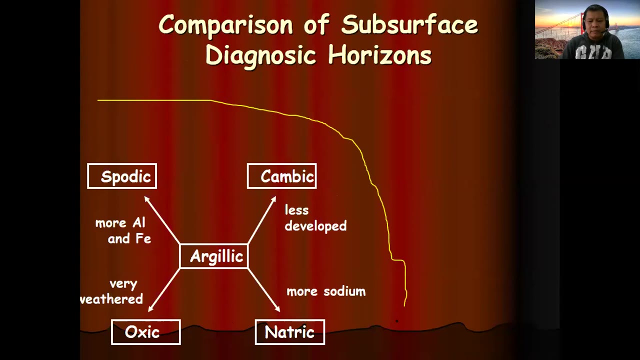 Then I will leave it on to you to read all of the diagnostic subsurface horizons. There are a lot of them, Okay anyway, So I'll just give you a copy for that. Okay, So this list will aid ourselves in memorizing the different subsurface diagnostic horizons. 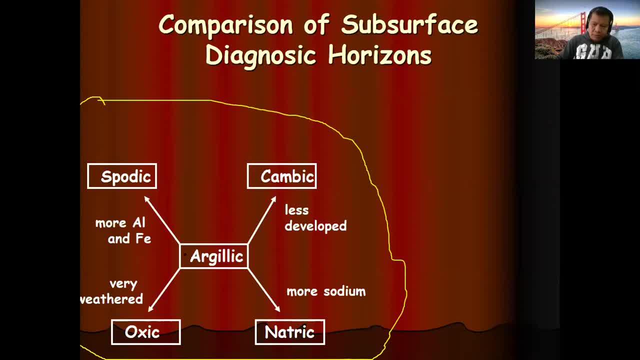 Okay, So the first thing you have to memorize is argillic: Compared to argillic, when it is less developed, then it must be cambic. Compared to argillic, if it has more aluminum and iron compared to argillic, it must be sputic. 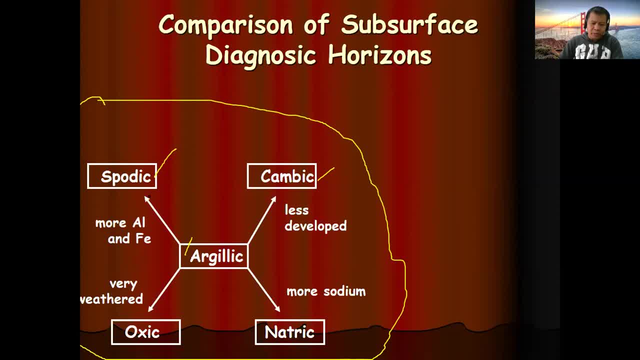 When it's very withered compared to argillic and compared to sputic, it must be an oxic diagnostic subsurface horizon Compared to argillic. if it has a natric more than 15% sodium It must be considered as a natric. 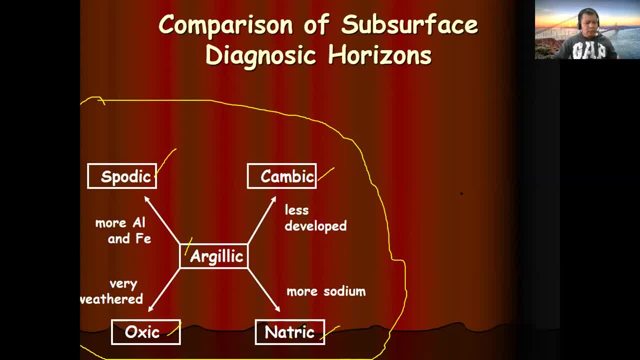 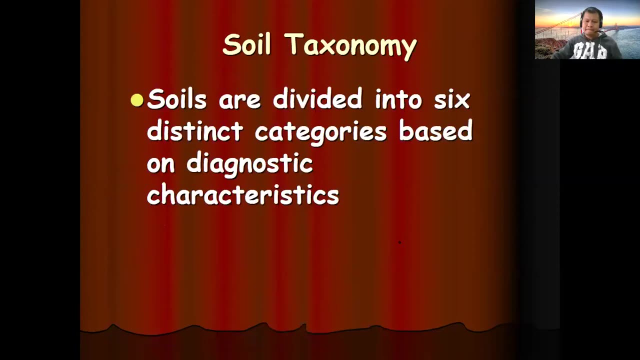 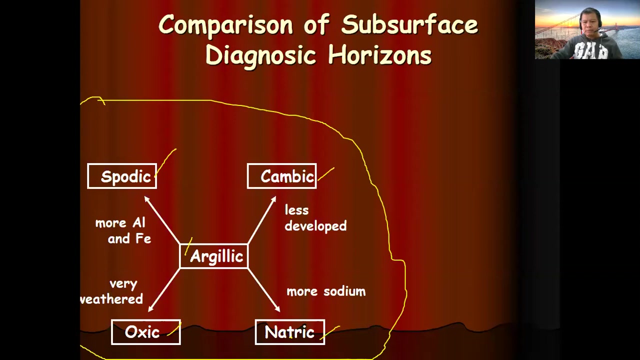 Okay, That is how we aid ourselves. we help ourselves in memorizing some of the diagnostic subsurface horizons that can be observed in the B or either in the C horizon. All right, So I guess we have to stop at this portion. 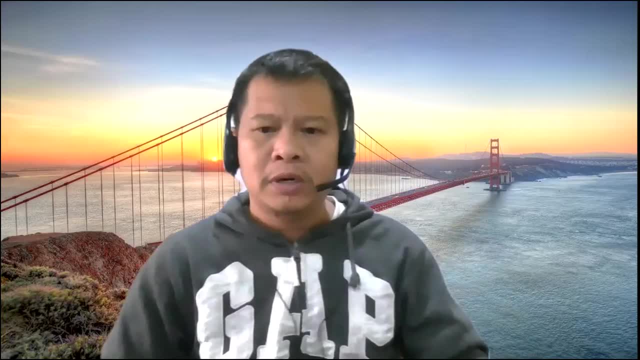 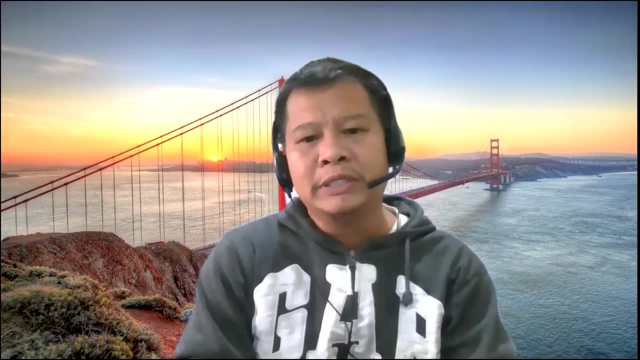 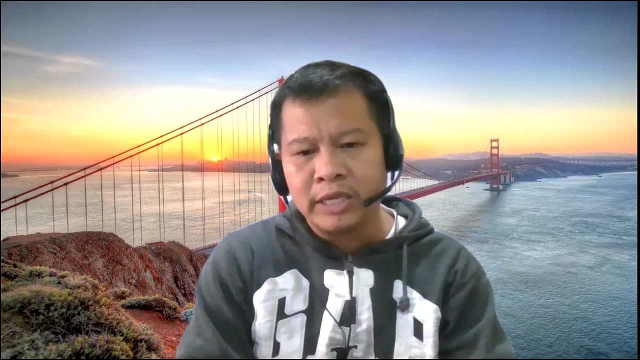 And then we'll proceed Later on on the succeeding topic And we can relax. We have different diagnostic horizons, We have the epipedons And the epipedons. we have mollic, ombric, ostic histic. 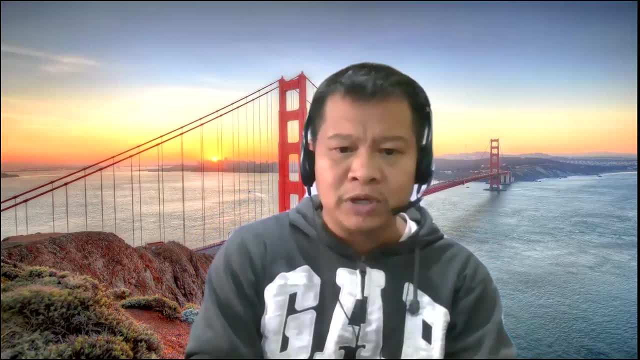 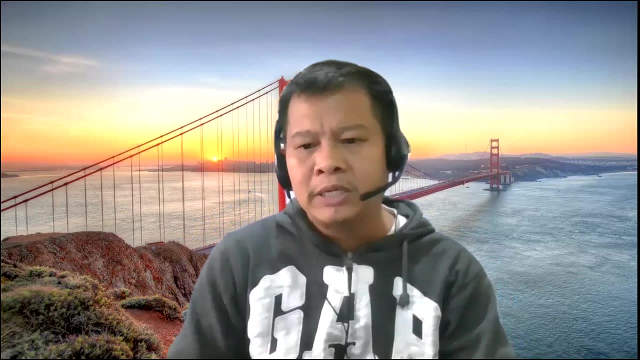 And we also have the diagnostic subsurface horizon that can be observed on the B horizon. We have the argillic natric, cambic sputic and many others. Okay, So I guess we have to stop After that.